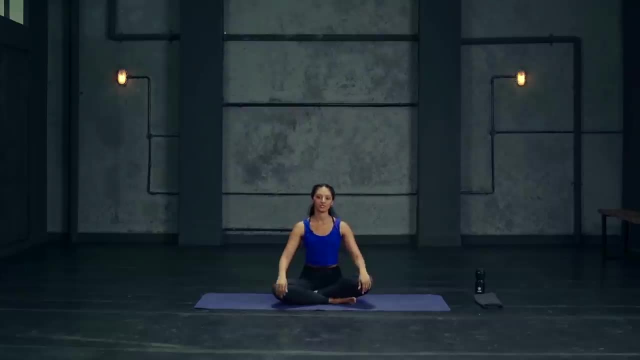 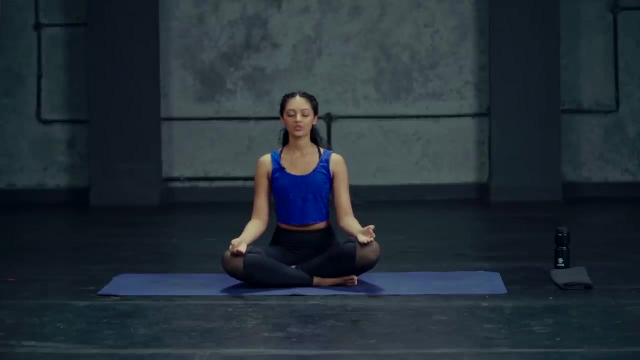 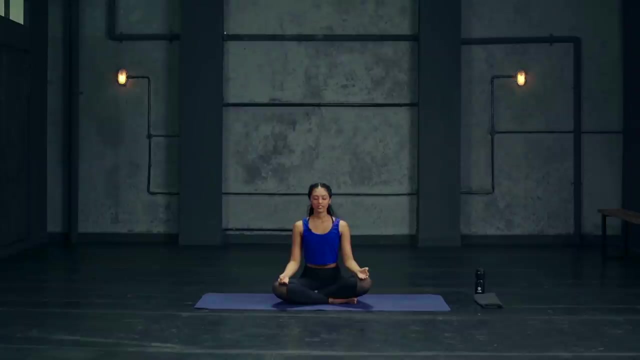 session for today. So come into any simple Sukhasana position. sit with your spine lengthened hands in Gyan Mudra or Chana Mudra, place it at your knees, roll the shoulders back and now slowly and gently close your eyes. Bring all the attention now onto your breath. 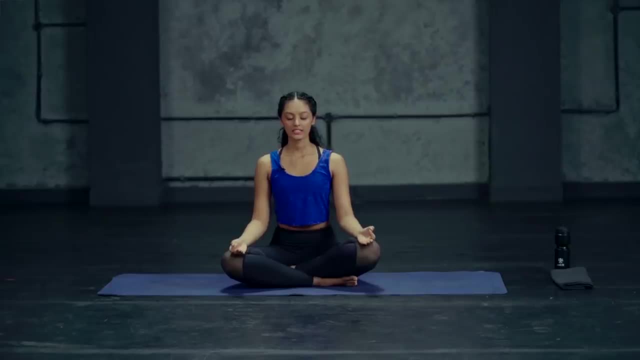 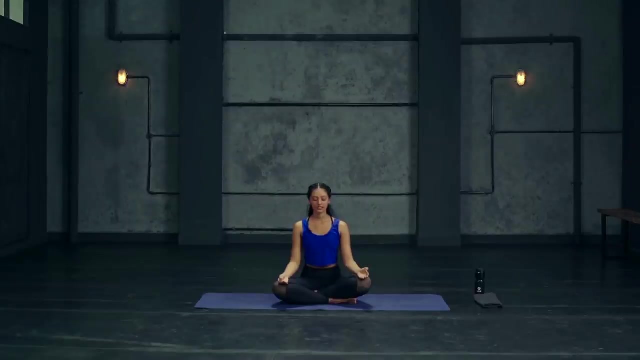 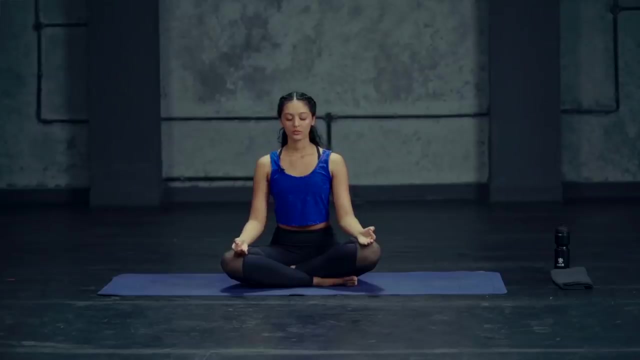 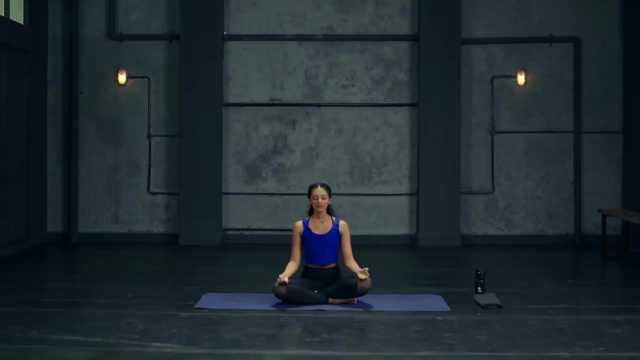 And inhale deeply And relax and exhale. Inhale once again And relax and exhale One more time A deep inhalation inwards And relax and exhale. And now focus on the quality of your breath, Experiencing the cool air entering your nostrils and the air. 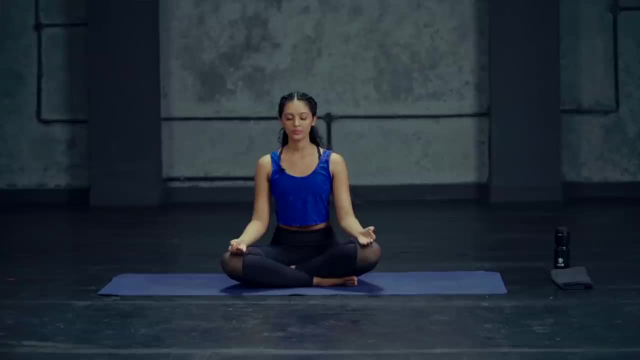 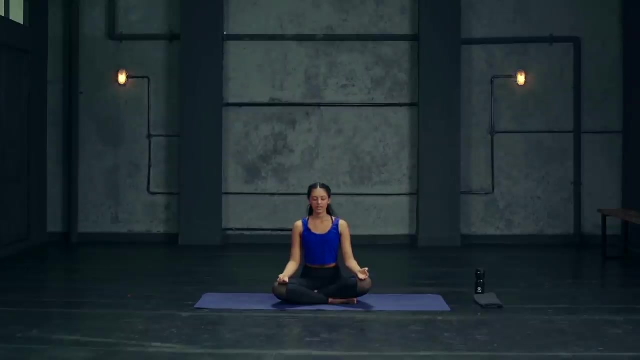 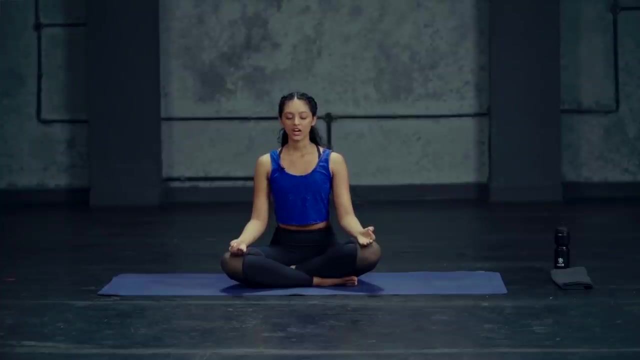 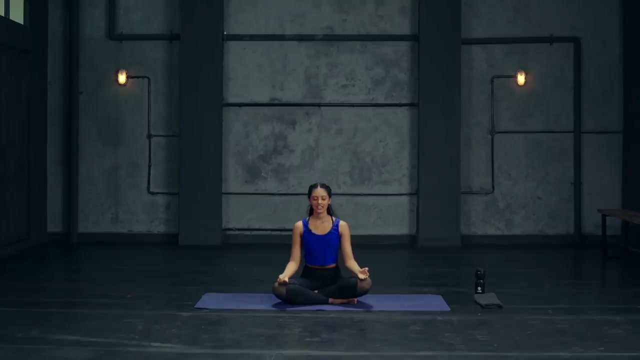 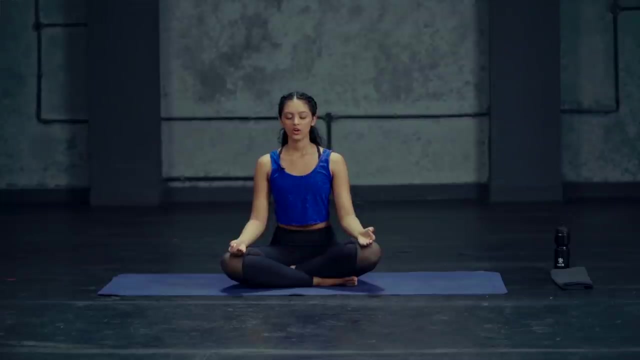 in yourMusic and the warm air gently leaving your nostrils And, as you do so, experience the deep sense of calm and relaxation, allowing your mind to completely be in the present moment. And now, just focus your attention on your mind, trying to observe your thoughts. 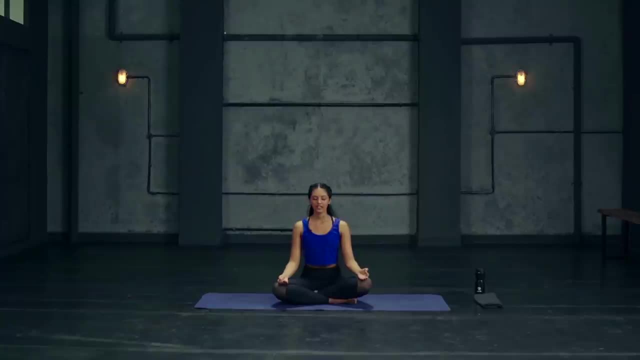 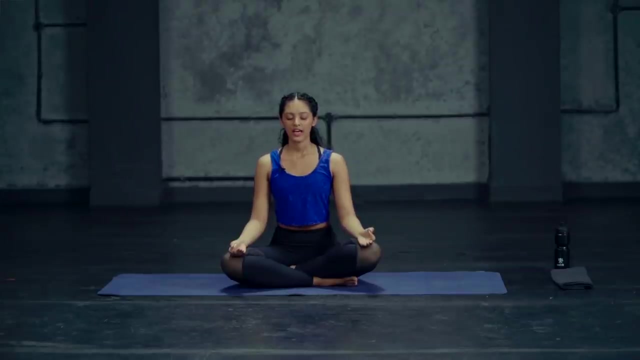 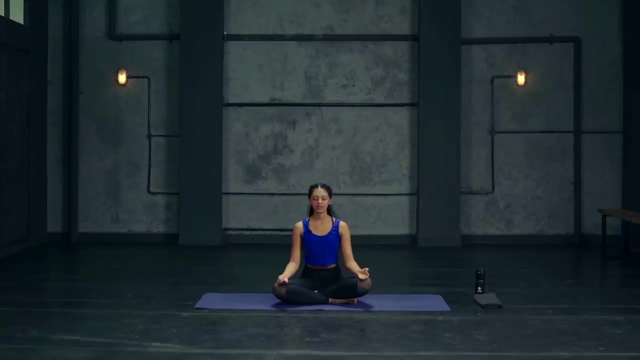 and trying to ground them even more in the present moment And now, as you've become fully aware of your breath and your mind, we're going to set a Sankalpa or an intention for today's session, which is to do every Asana and every practice. 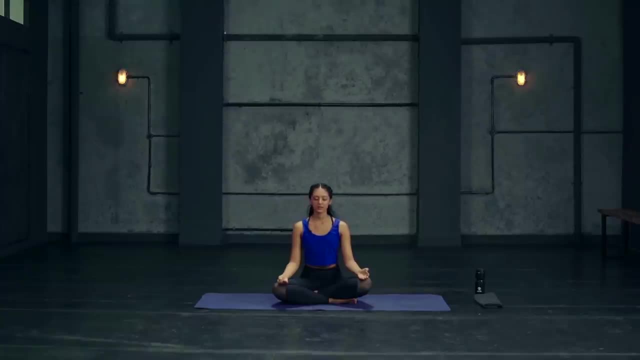 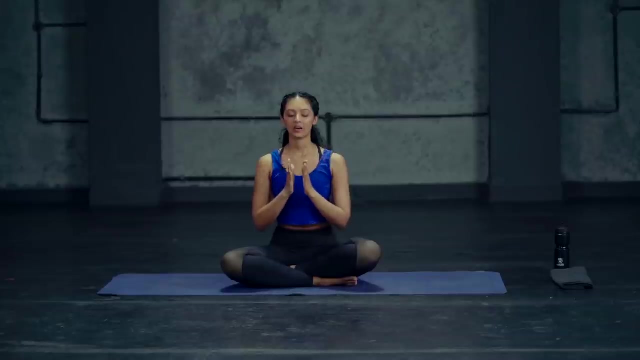 to the absolute best of our capacity. With that Sankalpa, bring your hands now into a Namaste at the chest. We're going to chant three short and sweet Om's together, So take a deep inhalation inwards now Inhale. 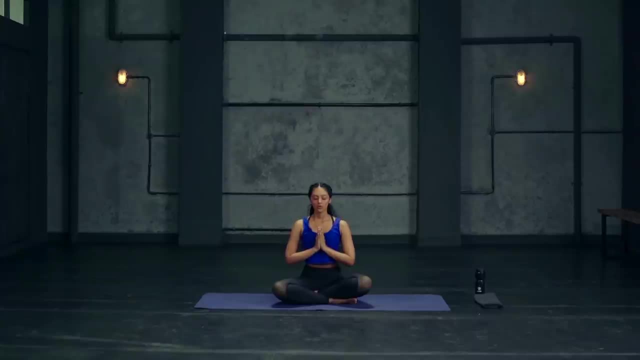 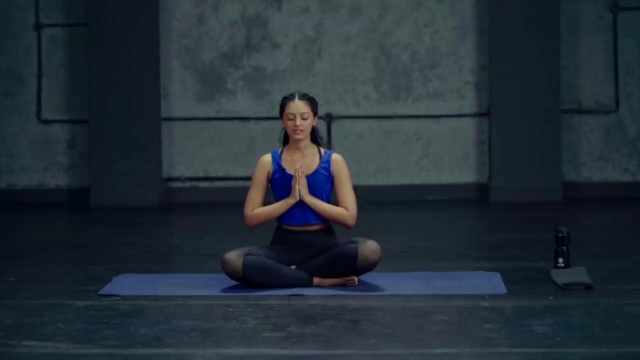 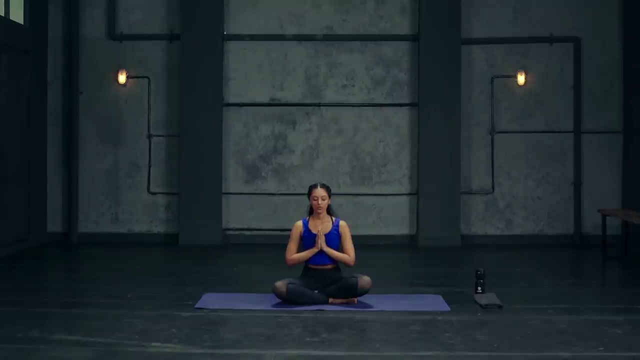 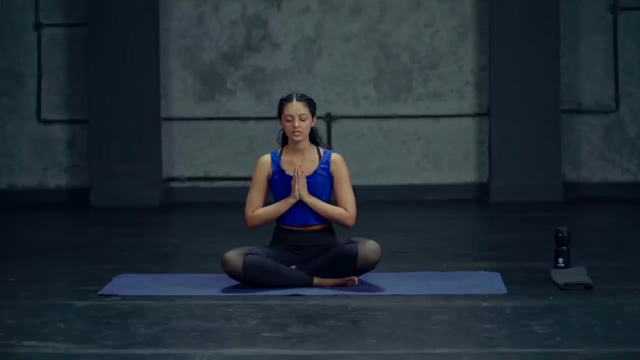 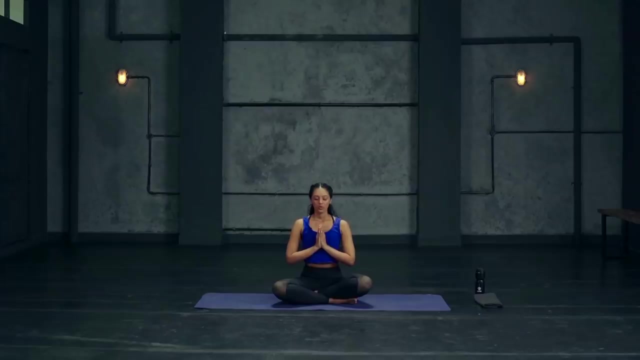 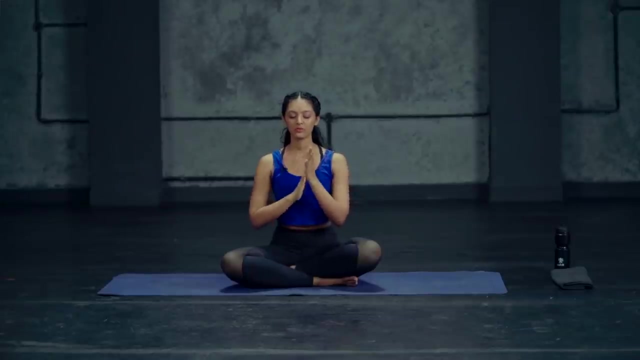 Om, Inhale once again Om And inhale one more time Om. And now, feeling that vibration of the Om, start to rub your palms together, creating some heat or friction, And place the palms on your eyelids, providing them with some warmth. 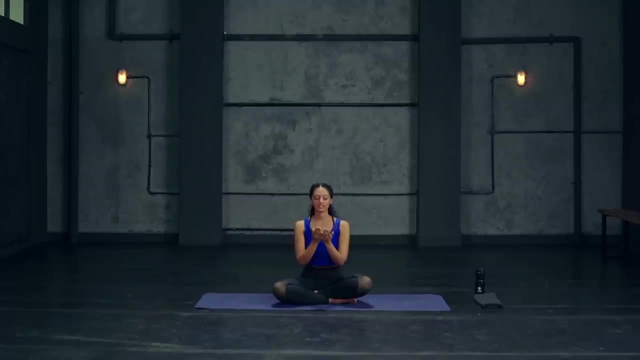 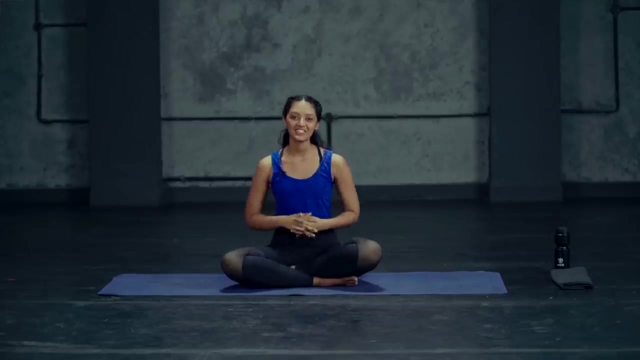 Rest of the face. Bring your hands down in front of your chest, Slowly open your eyes, Look at the palms, Bring the palms back and release. Fantastic. So that was our centering session for today. From here now we're going to get into our main practice. 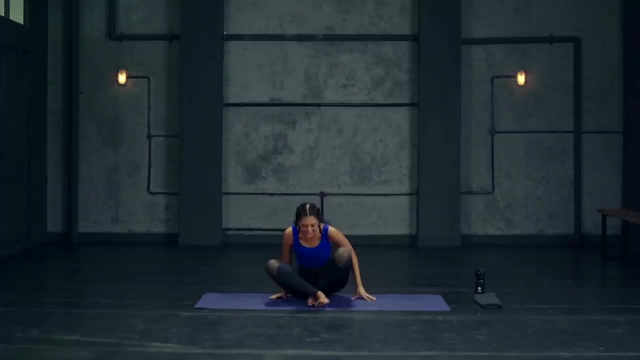 starting with the warm-up. So come into a standing position Now for the warm-up. I'd like to invite my fellow teacher, Gaurav, who's going to be demonstrating for us. So can we have, Gaurav? Thank you for being with us, Gaurav. 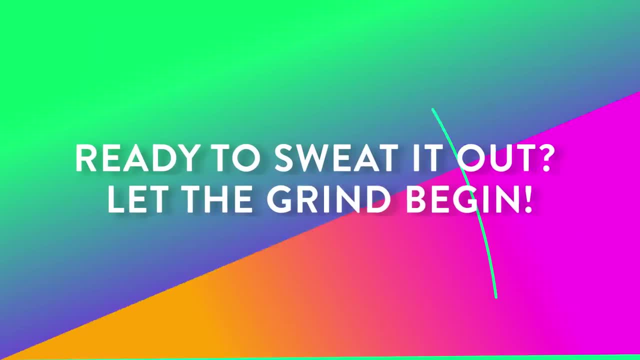 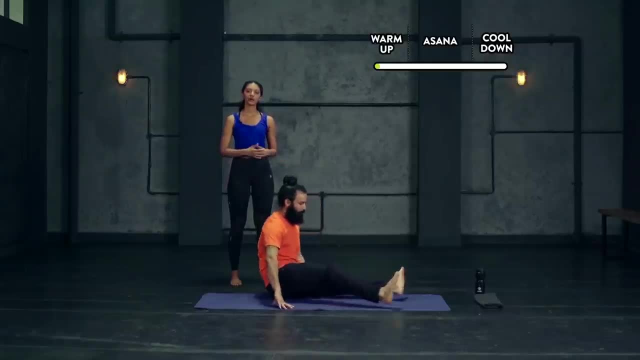 Namaste everyone. So we're going to start with a simple warm-up or a joint mobility movement. The first one is going to be in the sitting position So you can sit down on your mat. This is known as Chakki Chalan Asana. 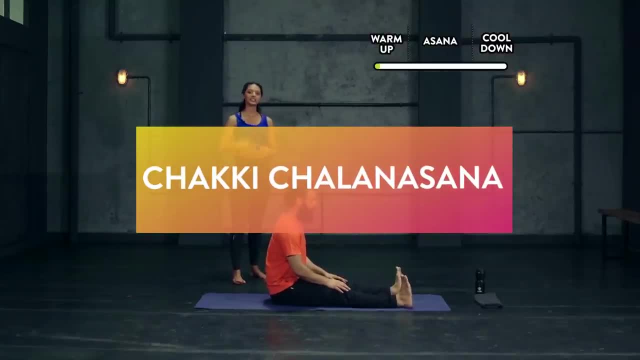 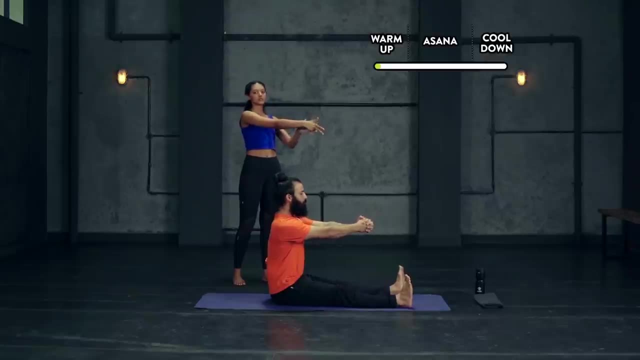 We're going to keep the legs hip-width distance apart, spine lengthened- sitting upright. Now bring your hands forward and interlock them together, keeping the elbows straight. We're going to inhale here And with the exhalation, bend forward completely. 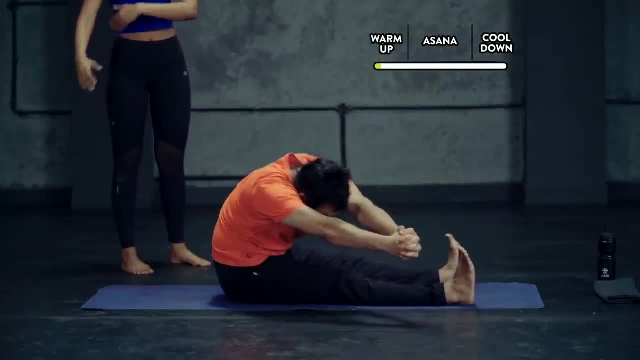 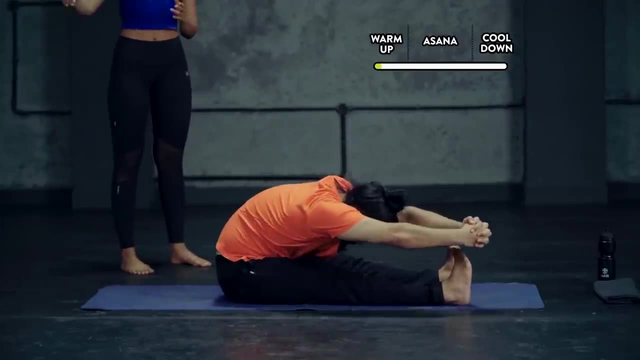 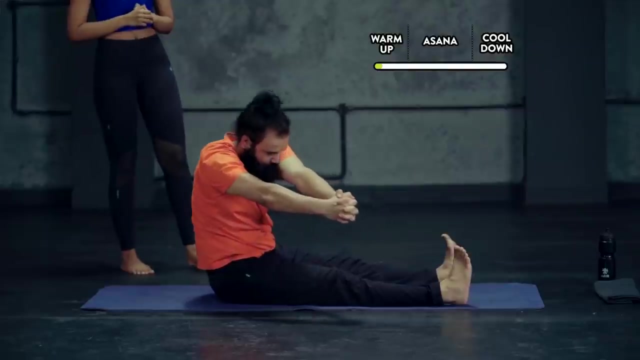 going all the way from the left foot to the right foot and back up, And then we'll repeat this five times. So repeat clockwise: left. all the way to the right, Inhale, Exhale and release going down, Come back inhale. 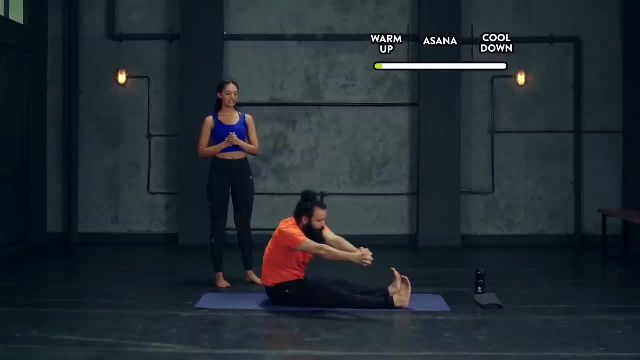 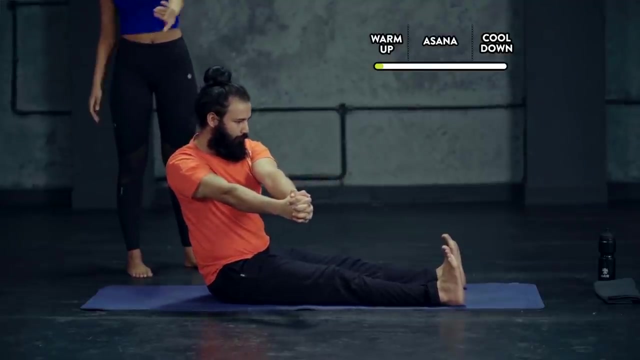 Exhale Left to the right toes, active Inhale And all the way down, Try and bring your head closer to your knees each time. And now we're going to go anti-clockwise, So sitting up straight exhaling. 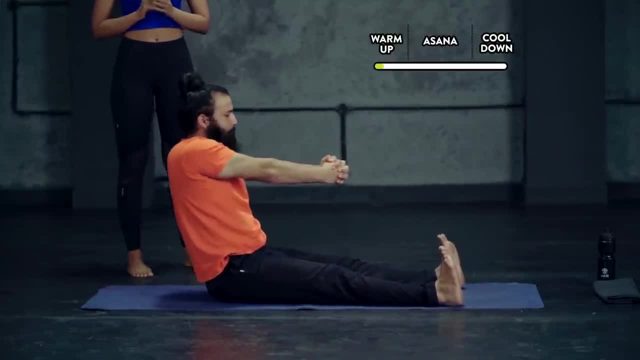 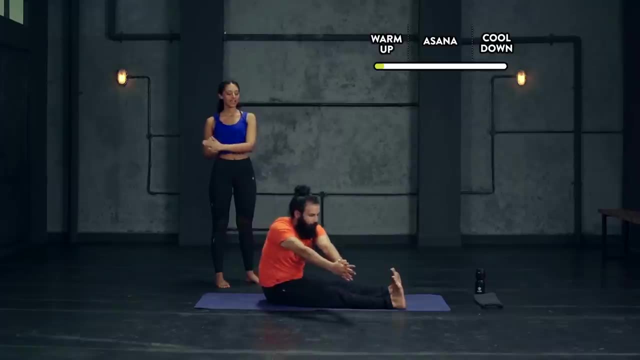 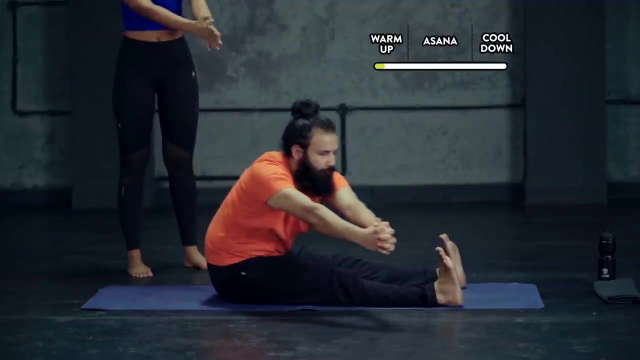 bringing your hands down from the right to the left. now Repeat second round all the way from the right to the left. Inhale at the top, Exhale, Bend forward, Come back And one more time going all the way down. 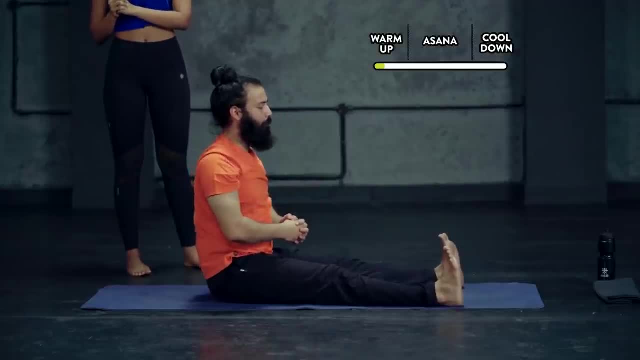 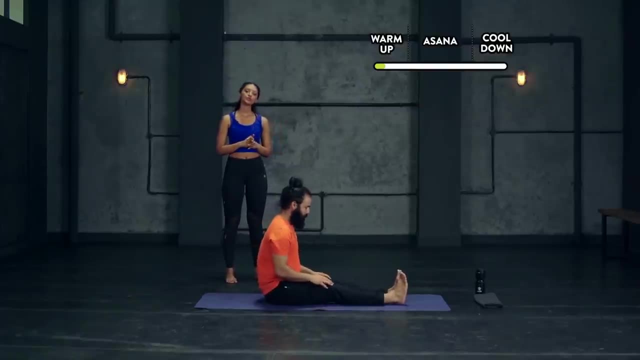 Release. You're going to feel tension releasing from your hamstrings on the back And back onto the mat- Brilliant. So that was our Chakki Chalanasana. We're also going to do a spinal twist here, just to make sure your spine is all warmed up. 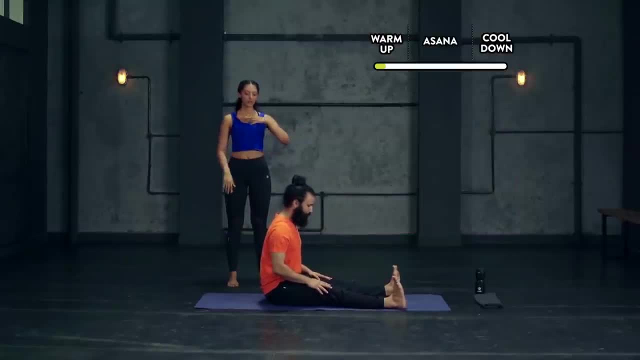 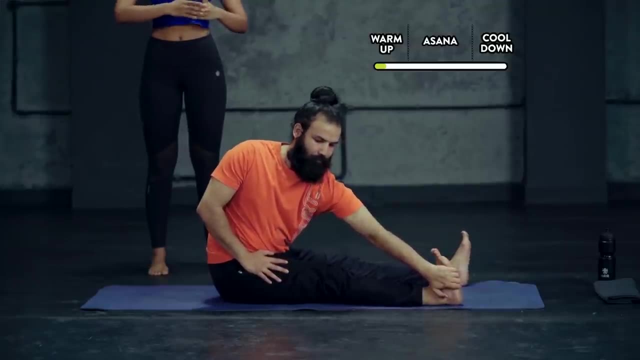 So now, keeping the legs hip-width distance apart, bring your left hand and place it in the arch of right foot. Once you've done that, you're going to open the chest out completely. Bring your right hand to the back and deepen the twist in this position. 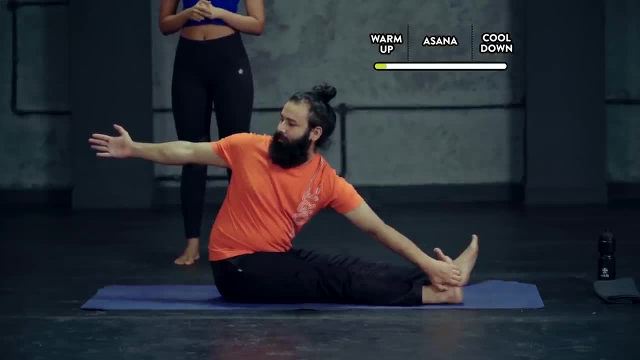 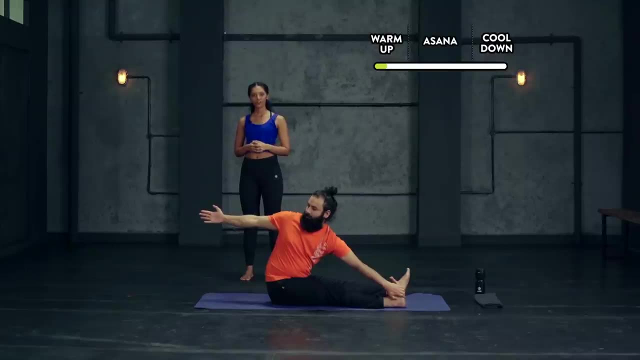 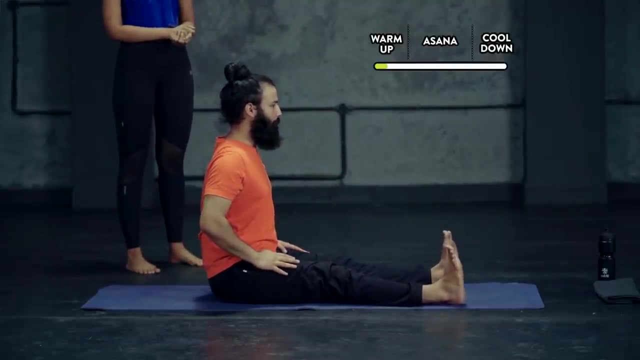 Hold here for five breaths: One, Two, Opening the chest out further Three, Four And five. Slowly bring the hand back, releasing the twist, Coming back to the central position. We'll repeat the same thing now, on the other side. 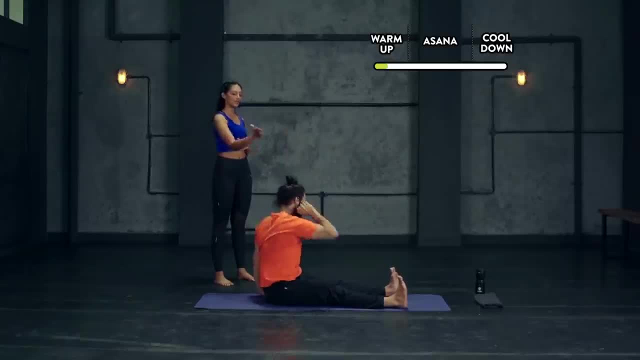 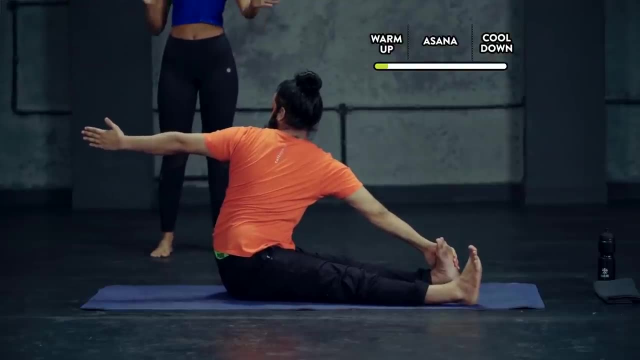 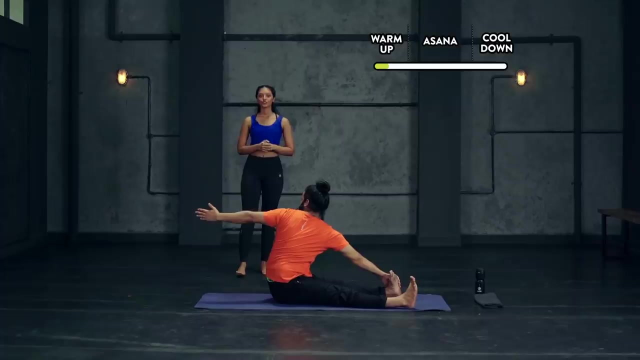 So take your right hand, bring it all the way onto the arch of your foot And, twisting, take the left hand outside, Completely twist your spine, Open out the chest and hold for five. One, Two, Three, Four And five. 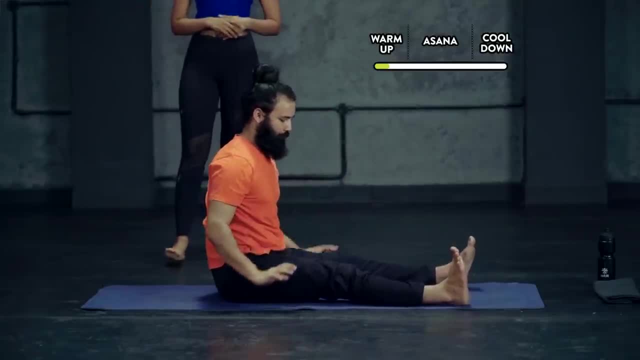 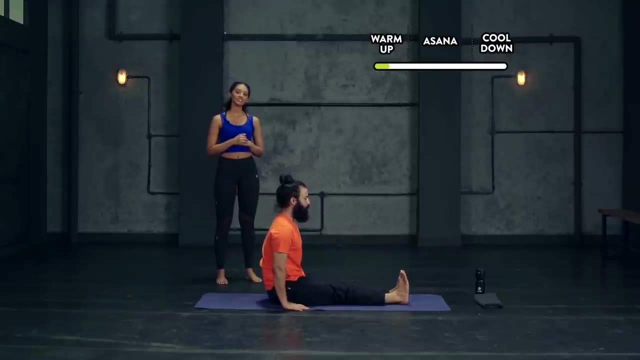 Now slowly come back, releasing the twist, Bring the hands back onto the mat. Brilliant, So that was our first joint mobility movement. Now we move to the second one, which is going to be a transitional movement. Let's learn how to practice this. 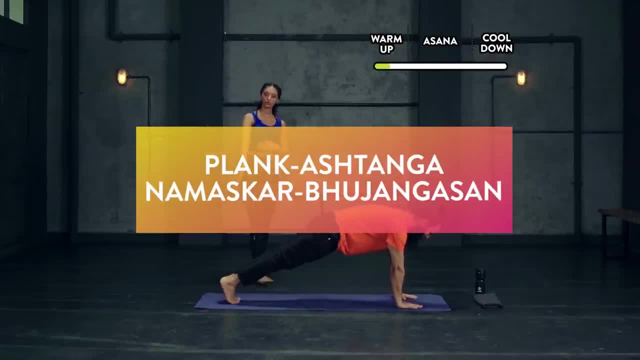 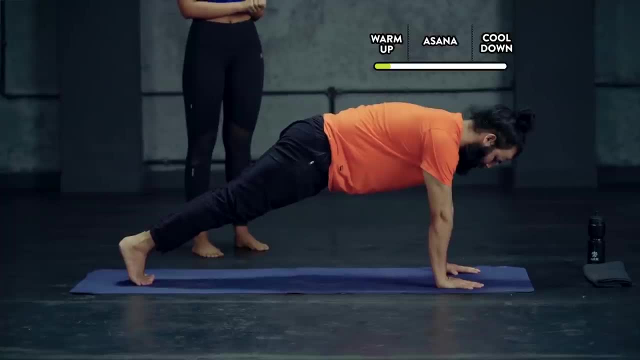 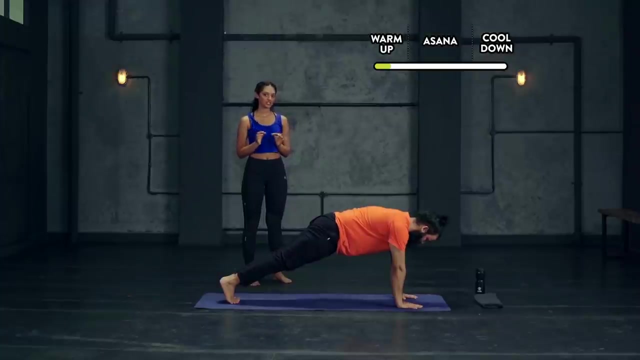 You first come into the plank position with your toes together at the back, heels and toes touching Hands forward. Make sure your elbows, wrists and shoulders are in one line and that your hips are not sinking downwards- Spine neutral. From here we're going to transition to Ashtanga, Namaskar. 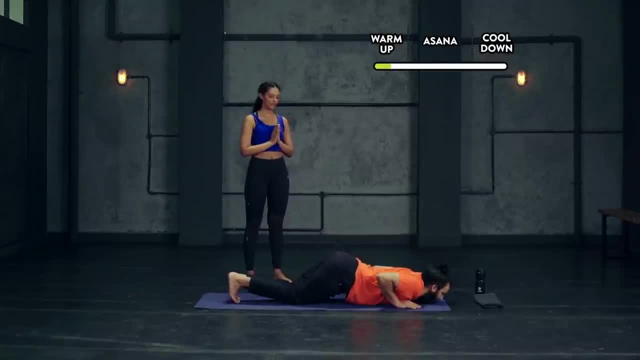 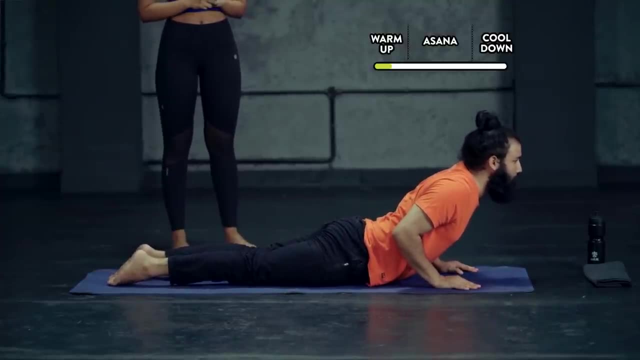 Knees, chest and chin on the mat. Brilliant, Now slide forward bringing the chest up, Inhale Toes flat at the back And then we'll repeat from plank into Ashtanga and Bhujanga- Five rounds. 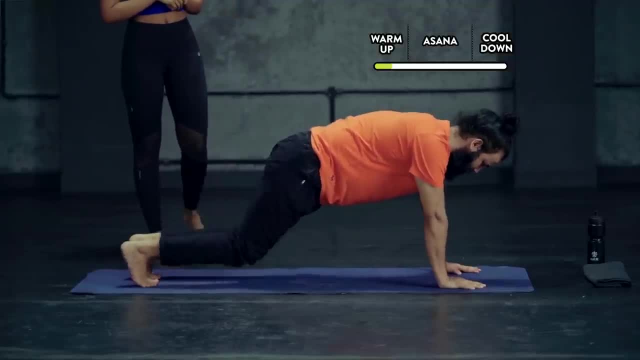 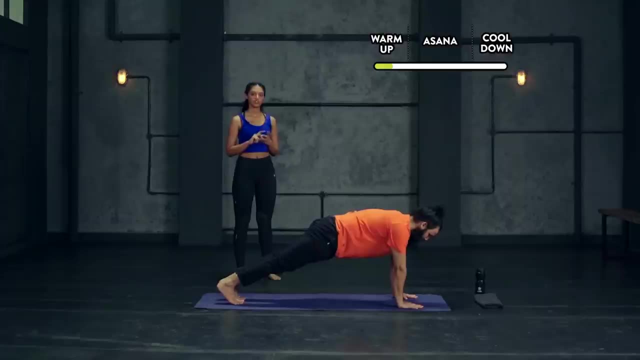 Let's begin round. one Plank Knees, chest and chin Ashtanga. Inhale Bhujanga And come back into plank Round two- Knees, chest and chin Ashtanga Namaskar. 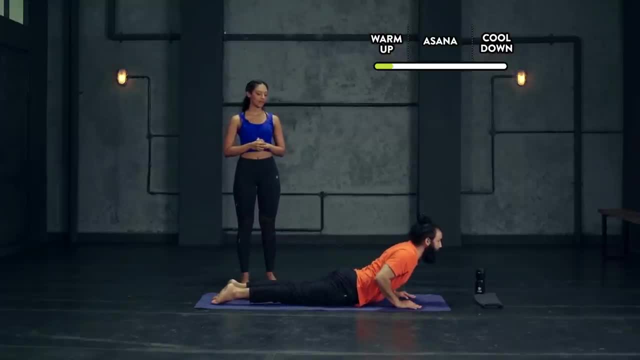 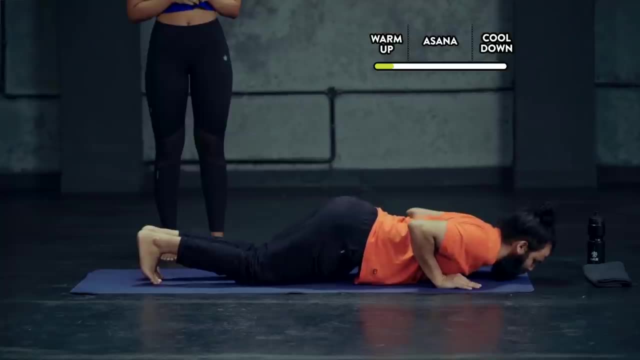 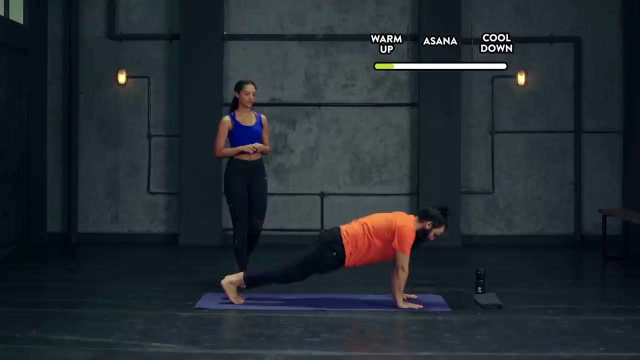 Inhale Plank, Sliding forward And come back into plank position. Now round three Knees chest and chin down on the mat. Now inhale, Slide forward into Bhujangasana And back into plank. 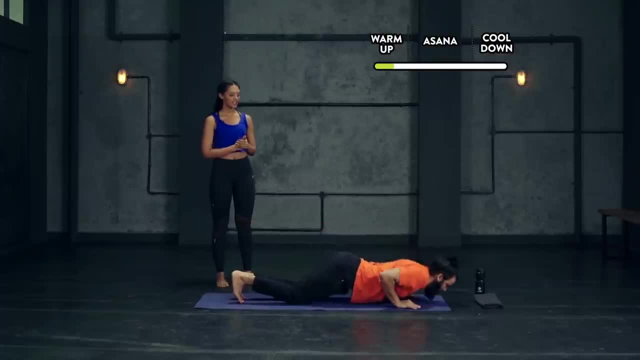 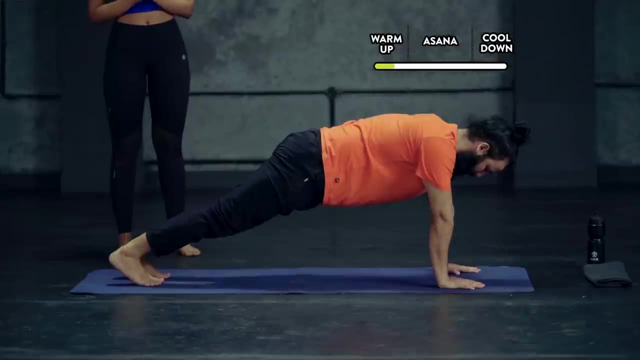 Round four: Knees, chest and chin, Sliding forward with the inhalation Bhujangasana And coming back into plank Last round: Knees, chest and chin on the mat. Inhale, Slide forward, Open the chest. 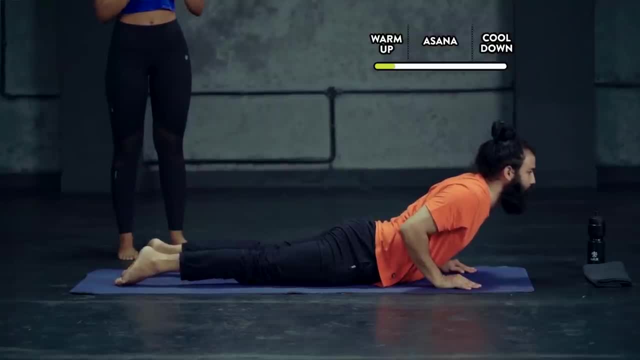 Bhujangasana. And now once again come back into plank. Fantastic. Now drop your knees down, Release the plank position, Beautiful. And now from here we are going to transition into our Surya Namaskar practice. So, coming on now to the top of your mat. 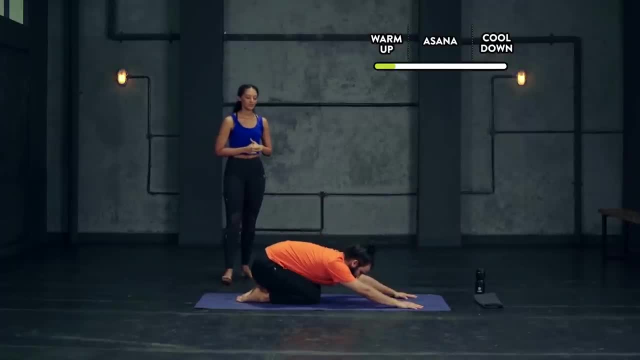 We're going to start with Ashtanga Surya, Namaskar A. Let's start with Ashtanga Surya, Namaskar A. Ashtanga Surya, Namaskar A. Let's start with Ashtanga Surya, Namaskar A. 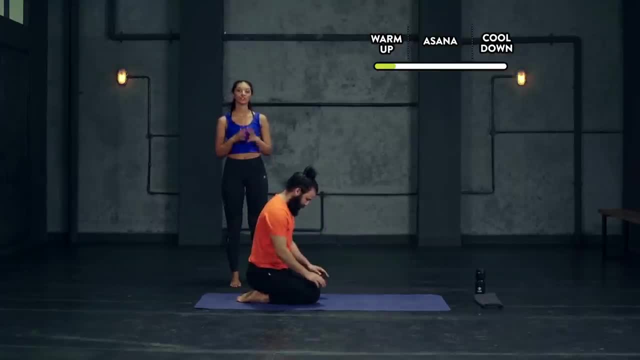 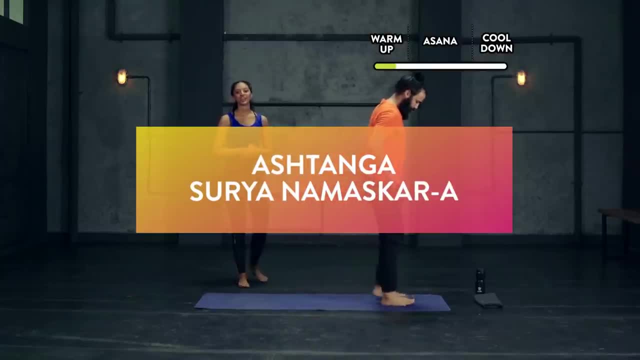 Ashtanga Surya, Namaskar A. Ashtanga Surya, Namaskar A. Let's begin this practice now. So now come into the Samasthiti position with your hands by the side of the body. Roll the shoulders back. 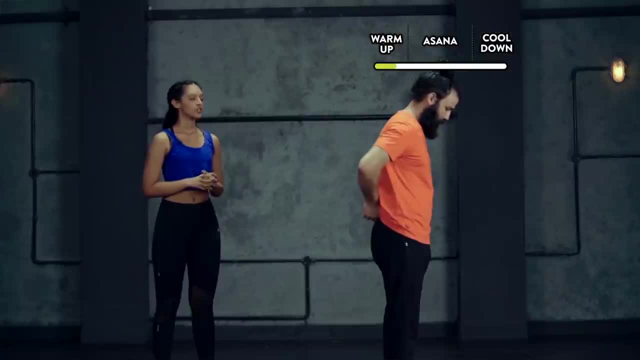 Tailbone tucked in, Kneecap pulled up. And now we're going to start with the first position, Bringing your hands all the way up, Taking it as close to the ears as possible, Hands and ears in one line. Lengthen the spine and knees. 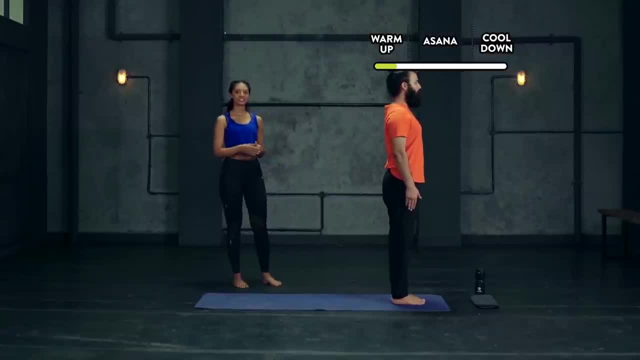 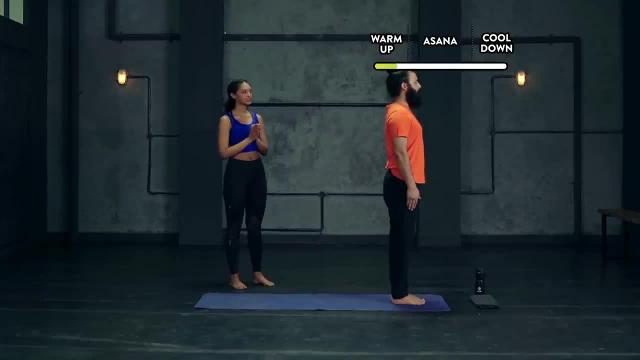 abs pulled up. and now we're going to start with the first position, bringing your hands all the way up, taking it as close to the ears as possible, hands and ears in one line. lengthen the spine and inhale here. now exhale, bend forward from the hips, coming all the way down. 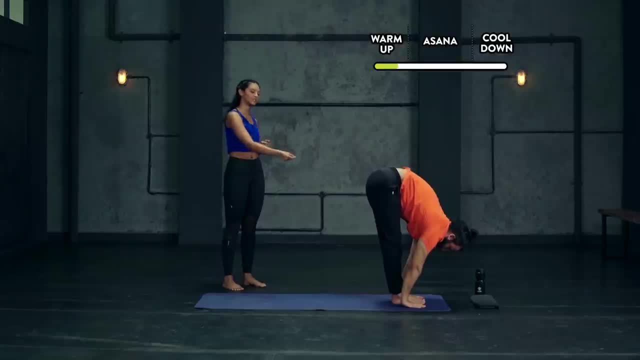 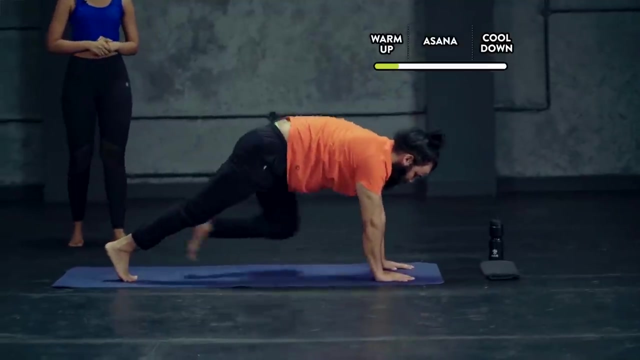 placing your palms on the mat. if you're finding this challenging, you can keep the knee softly bent, but if you're fine, then keep the knee straight now. fingertips on the mat- inhale. look forward from here. palms on the mat once again, exhale. jump or walk back into chaturanga. 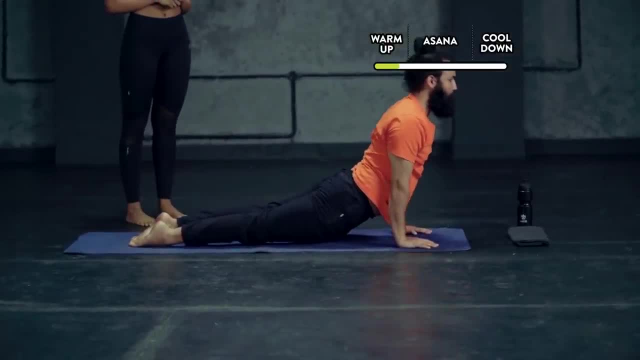 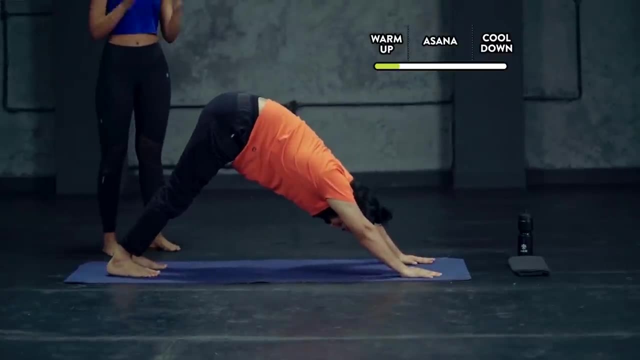 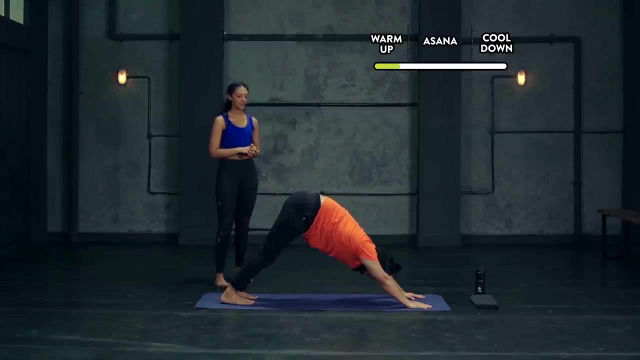 from here: inhale urdha mukha upward, facing dog, toes flat at the back, and exhale adho mukha downward, facing dog, over here. we're going to take five breaths- one, two, three, four and five- and now walk or jump back with the feet between the palms, ardha uttana fingertips on the mat. 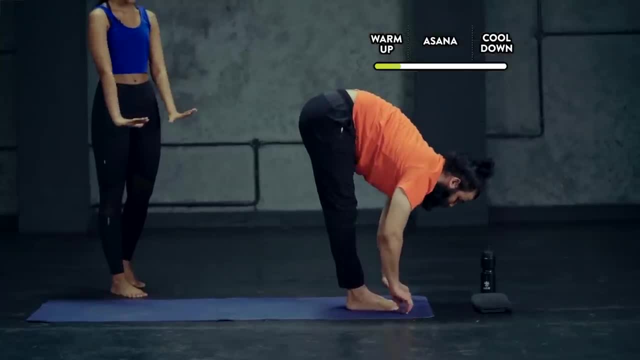 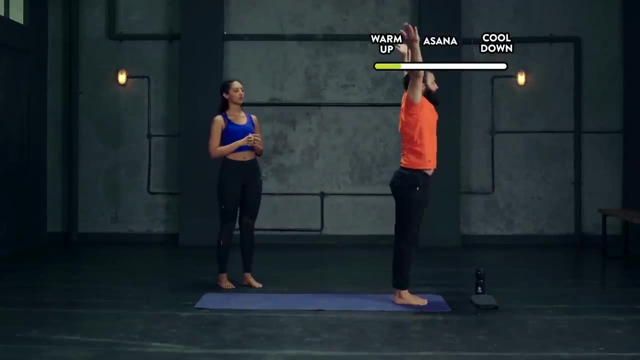 looking forward. spine neutral and now uttanasana, palms flat on the mat with the exhalation inhale, bring the arms up, coming all the way to the top, hands close to the ears and slowly bring the hands back down into samasthiti. brilliant, so that is one round of ashtanga. 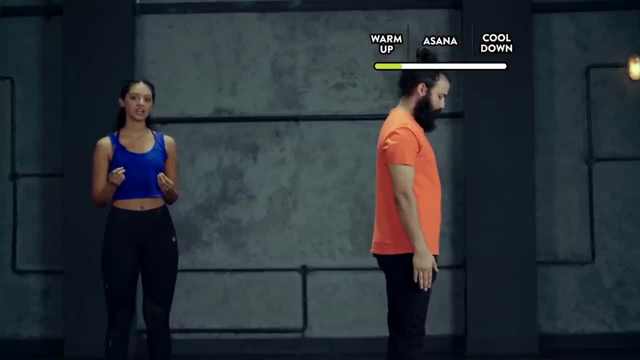 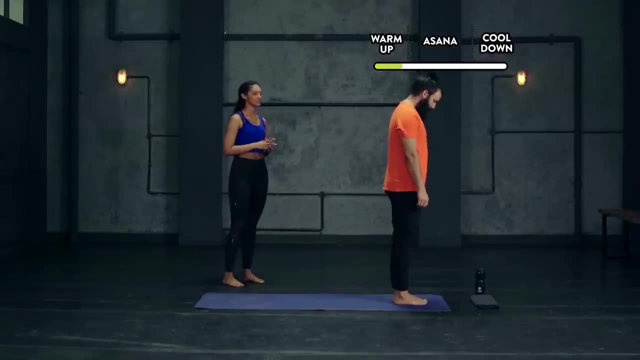 sir namaskar a, we're going to do two and three a little faster now, and then we're going to try and increase the challenge as we keep getting deeper into the surya namaskars, let's begin so, samasthiti, roll the shoulders back, stand straight now, inhale, take the arms up, lengthen the spine as. 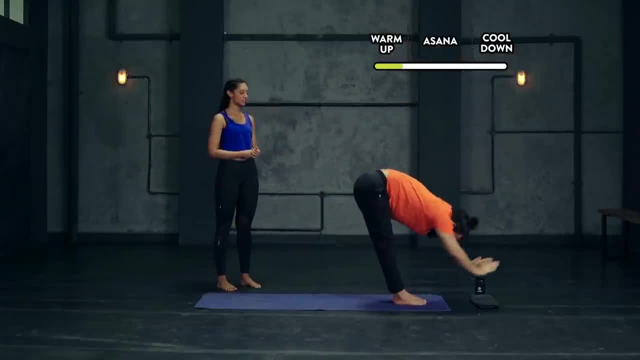 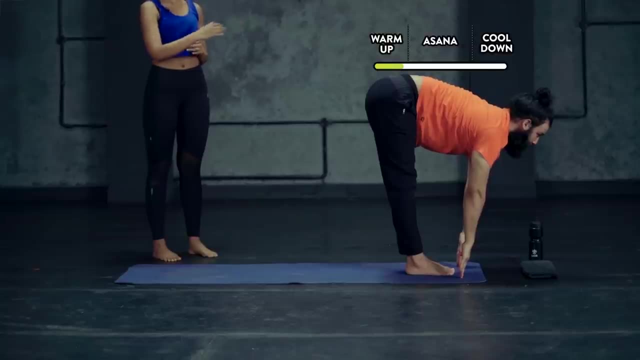 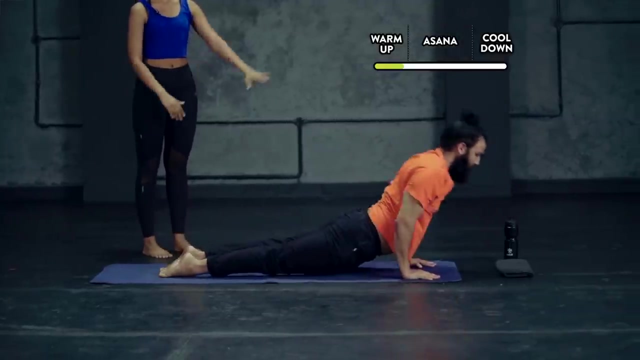 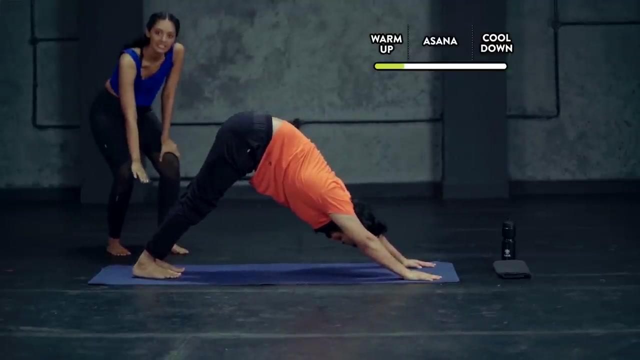 much as you can exhale. bend forward from the hips. uttanasana, palms flat. inhale ardha uttana fingertips on the mat looking forward, palms on the mat- exhale. jump back into chaturanga. inhale. slide the chest forward, urdhamukha. 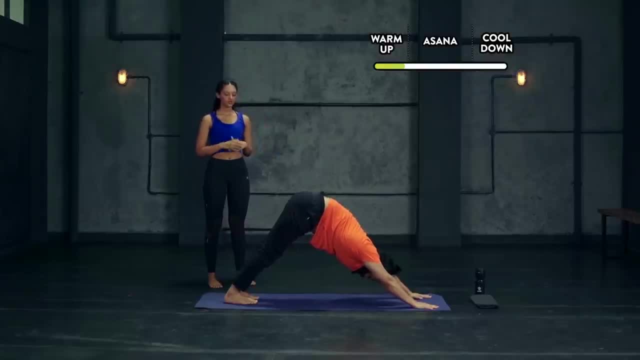 exhale. come onto your feet, adhomukha. try and bring the heels down if possible to really deepen the stretch in this position. hold for five: one, two, three, four and five. now walk or jump back with the legs in between the palms. ardha uttana inhale. look forward, uttana exhale. 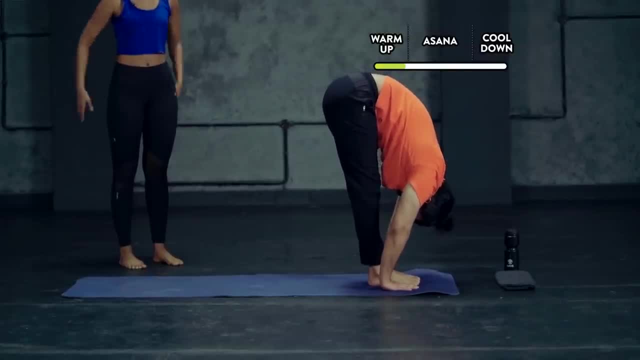 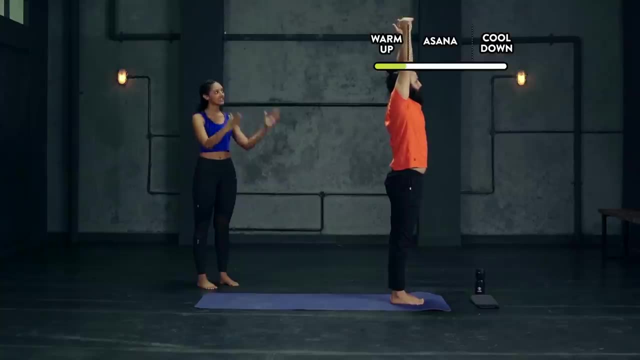 limb moves up. fold knee, nope, liberated lightly. knees gracely bend이 sweetheart highness. Exhale. Palms on the mat, Knees straight. Inhale. Come all the way to the top. Urdhva Hastasana, Hands close to the ears. Exhale Back down into Samasthiti, Third round, Going straight from here. Inhale Arms up. Urdhva Hastasana, Exhale Bent forward. Uttanasana Palms flat on the mat. Inhale. Ardha Uttana, Fingertips on the mat, Look forward. 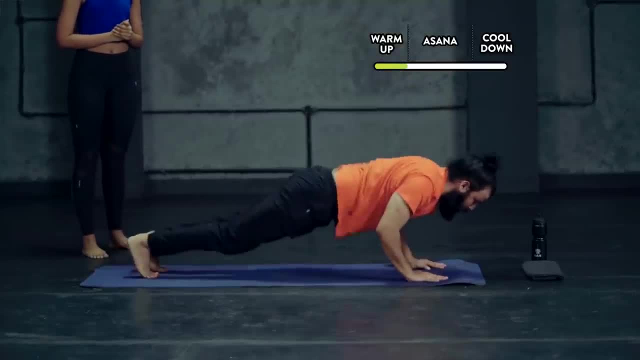 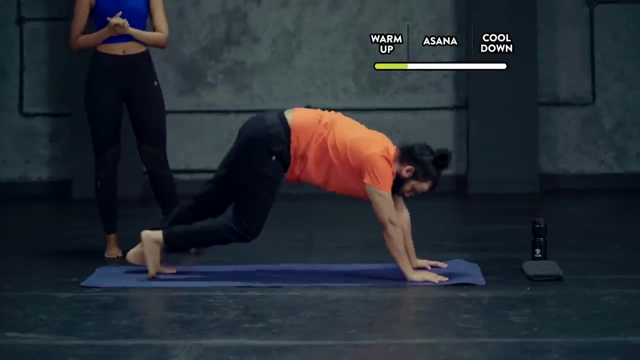 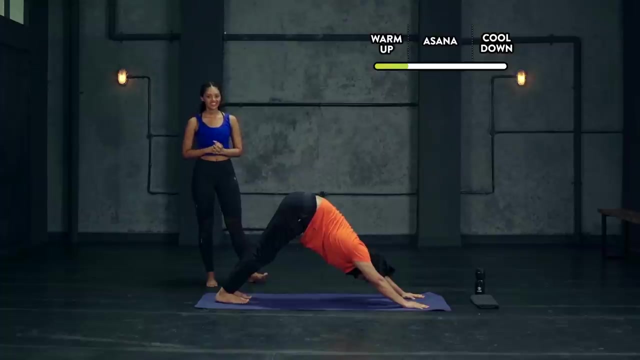 Jump back now into Chaturanga. Fantastic Now inhale. Slide forward Urdhva Mukha, Exhale Adho Mukha. Heels on the mat, Hold for 5.. 1,, 2,, 3,, 4 and 5.. 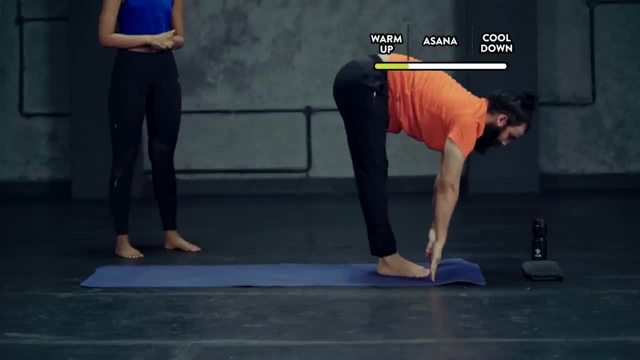 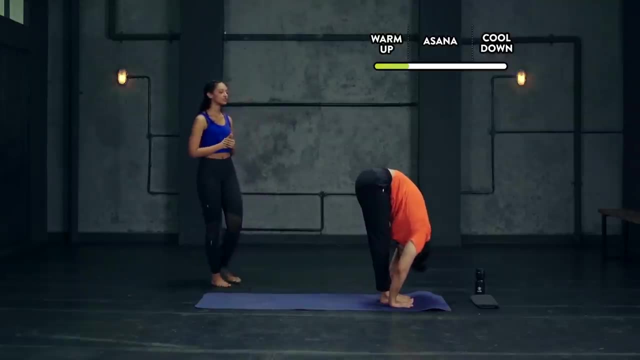 Now jump forward. Legs between the palms, Ardha Uttana- Inhale. Exhale Uttanasana. Palms on the mat: Inhale Urdhva Hastasana All the way to the top, Palms up, Hands close to the ears. Exhale Samasthiti once again. 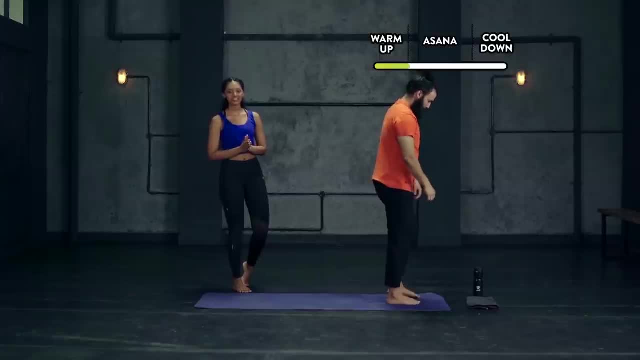 Brilliant, Beautiful. So that was our Surya Namaskar practice. Now we need to take some rest for a few moments. So keep a little distance between your legs, Hands open, Palms facing the front, Let your armpits breathe and just relax here for a few seconds. 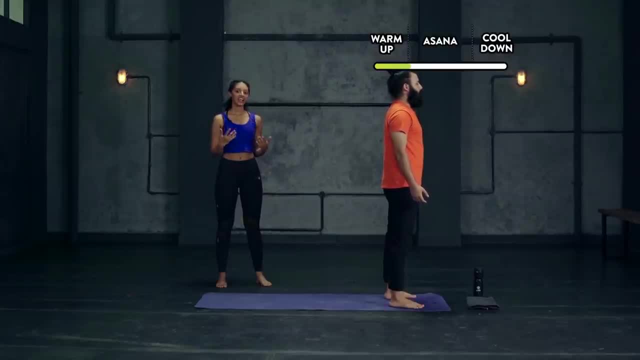 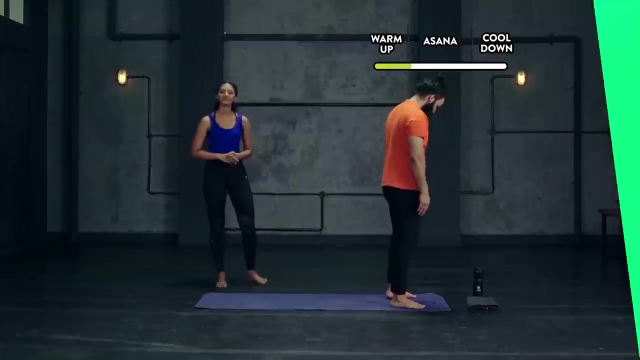 Inhalations inwards And relaxing with the exhalation. So you've all done a fantastic job with Surya Namaskar And we're going to get into our main sequences now, Just taking that little rest before we do so. Alright, let's begin. So we're going to start with sequence 1.. The way we start sequence 1 is we lead you into Adho Mukha, So just follow our instructions. 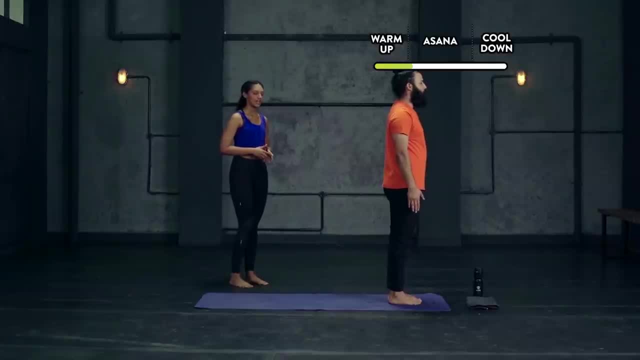 Standing in Samasthiti. now Roll the shoulders back. Now bring yourself into Utkatasana, So inhale Arms up Utkatasana. Now exhale Uttanasana, Bending forward Ardha Uttana with the fingertips on the mat. 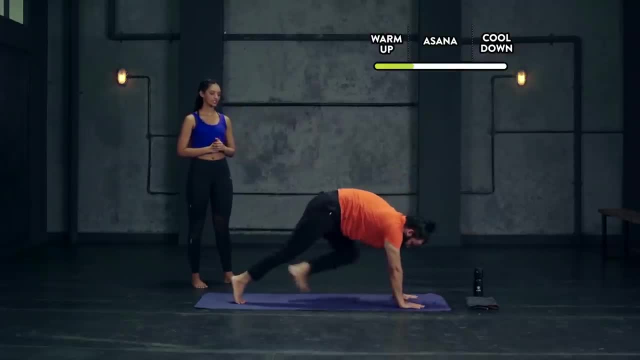 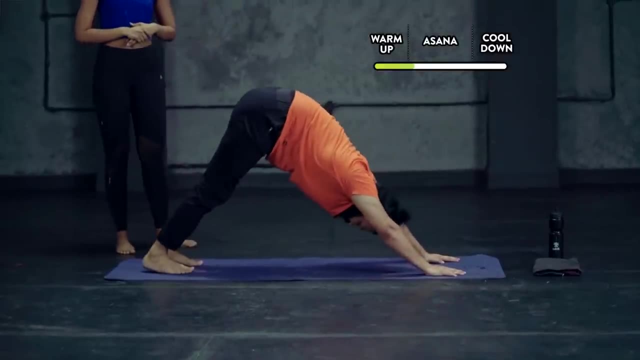 Walk or jump back into Chaturanga. Legs back, Inhale Urdhva Mukha And exhale into Adho Mukha. Alright, so this Adho Mukha is going to be our starting position. This first sequence is Adho Mukha. 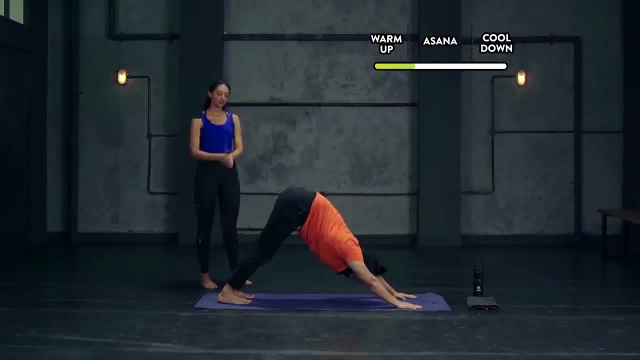 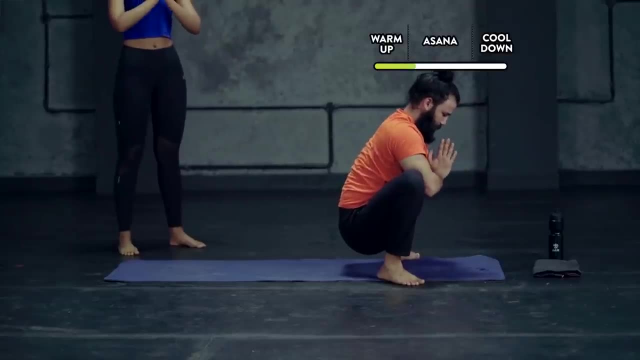 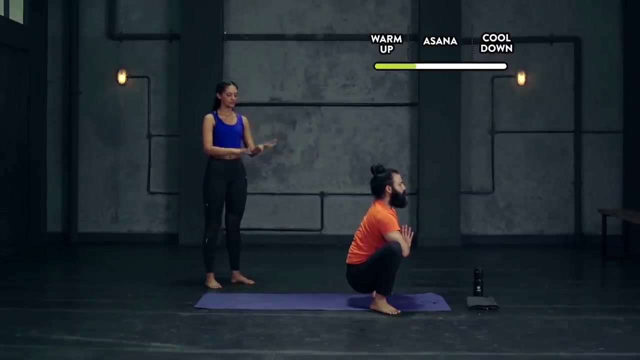 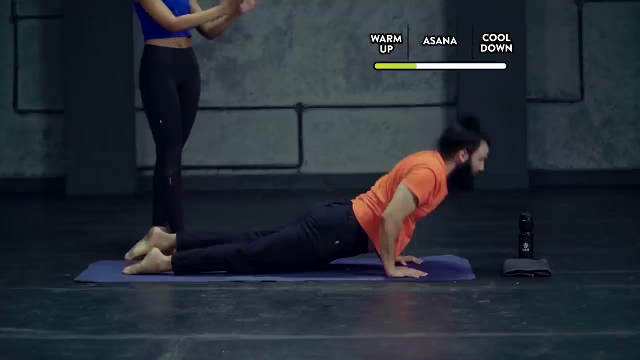 To Malasana. Let's begin From Adho Mukha. jump forward with the legs outside the palms into a Malasana. Now bring the palms into a Namaseth chest. Use the elbows to take your thighs outwards a little more. Now palms flat on the chest. We're going to take a Vinyasa here. Jump back into Chaturanga. Urdhva Mukha- Inhale. Adho Mukha, Exhale, And now round 2.. 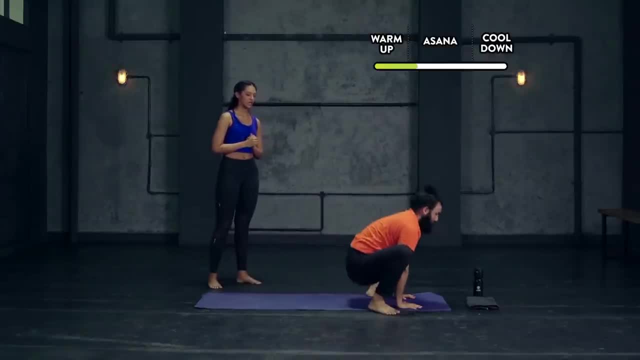 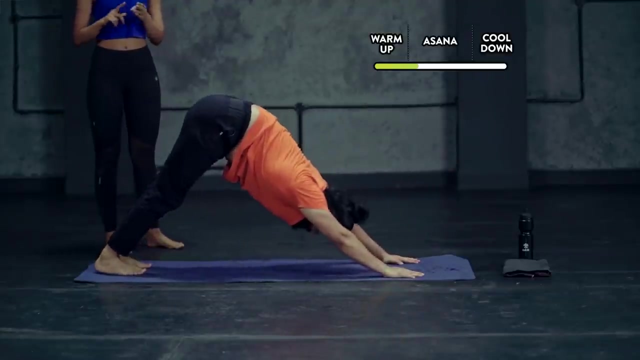 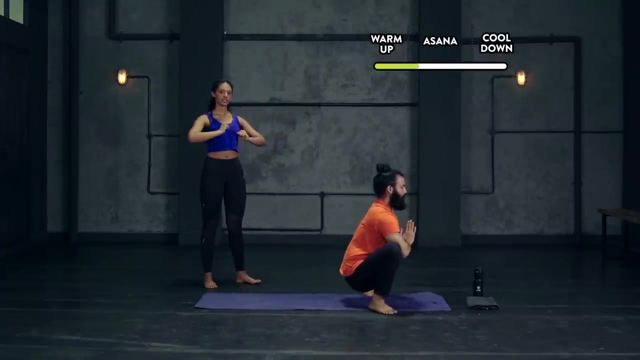 Jump back into Malasana Legs outside, Palms at the chest, Namaste. Now place the palms back on the mat. Chaturanga Legs back. Jump back Urdhva Mukha- Inhale Adho Mukha, Exhale From here round. 3.. Jump forward into Malasana Legs outside the hands, Namaste at the chest. Use the elbows to push out. Now place the palms on the mat once again And jump back into Malasana Legs outside Palms at the chest, Namaste. Now place the palms back on the mat, Chaturanga Legs back. Jump back Urdhva Mukha- Inhale Adho Mukha, Exhale From here round. 3.. Jump forward into Malasana Legs outside the hands, Namaste at the chest. Use the elbows to push out. Now place the palms on the mat once again And jump back into Malasana Legs outside the hands, Namaste at the chest. Use the elbows to push out. 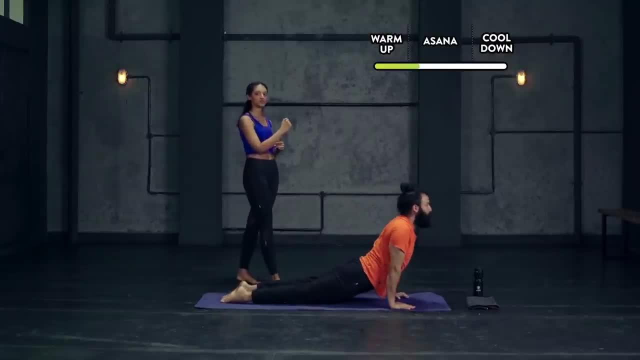 Chaturanga Urdhva Mukha. with the inhalation, Exhale Adho Mukha And now, round four, Jump forward into Malasana, once again Keeping the legs outside Namaste at the chest Spine. 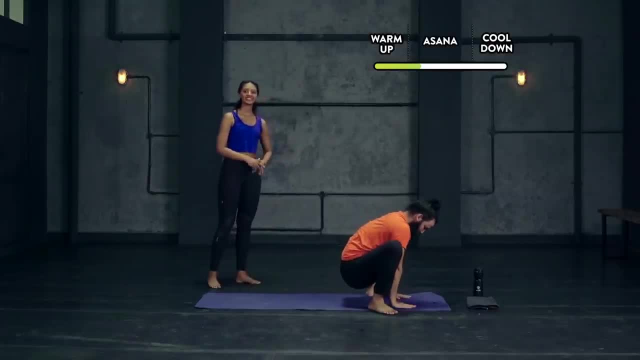 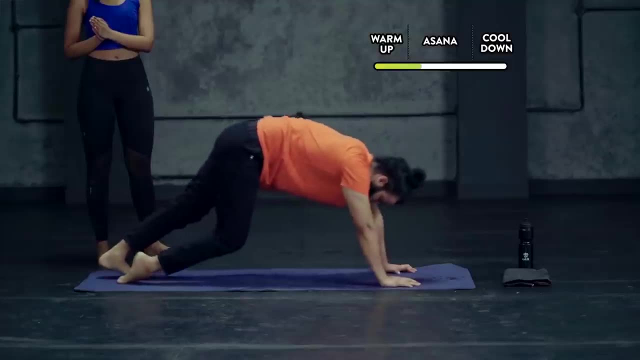 straight. Now palms on the mat, Release and jump back into Chaturanga. Urdhva Mukha Inhale. Adho Mukha Exhale. Now round five, Jump forward into Malasana once again, Legs outside. 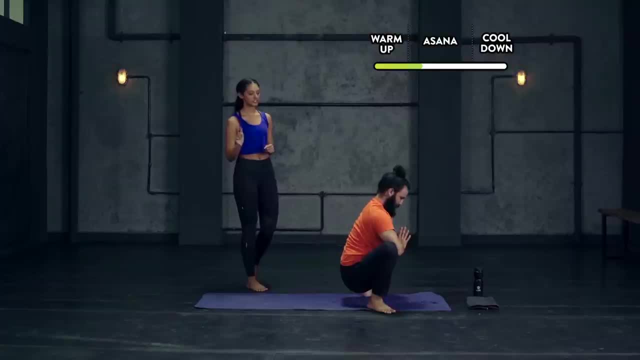 Palms at the chest. This we will hold for five breaths: One, Two, Three, Four And five. Release the palms, Place them on the mat once again, Jump back into Chaturanga. Urdhva Mukha. 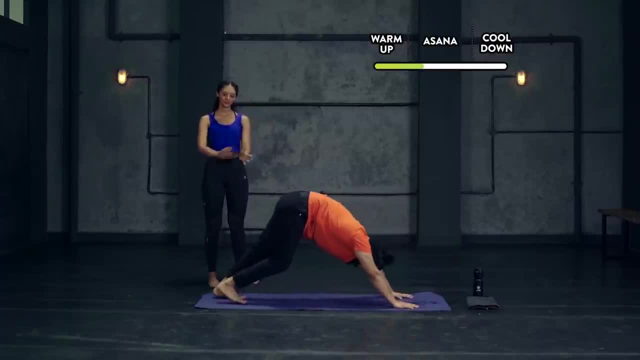 And Adho Mukha. Now back into Adho Mukha Asana. So this is now our starting position for sequence two. If you need to take some rest here, please drop your knees down, Come into a simple child's pose And just relax here for a few seconds. Our second sequence. 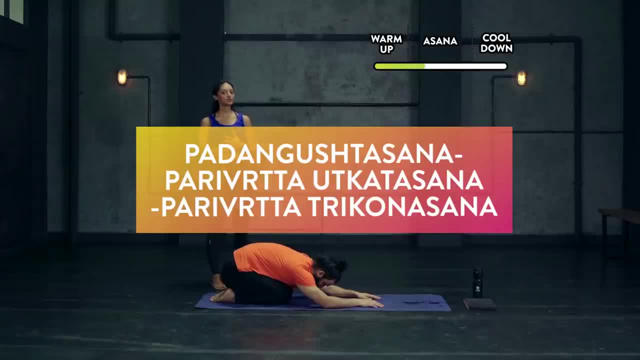 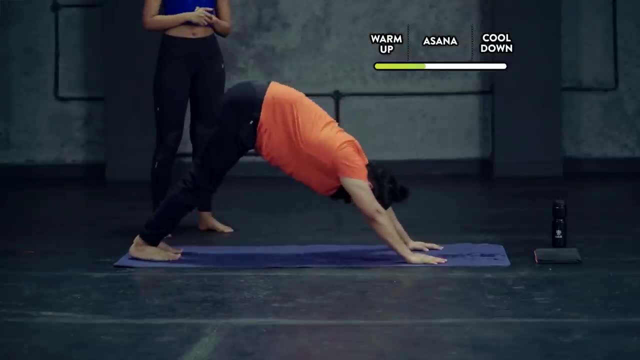 now is going to be Padangushthasana to Parivritta Utkatasana and then Parivritta Trikonasana, So let's learn how to practice this Transition now into Adho Mukha Svanasana once again. 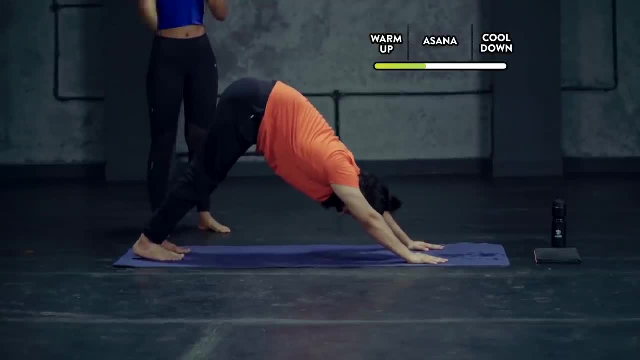 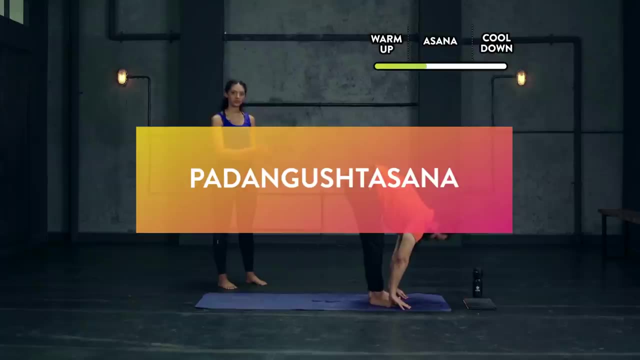 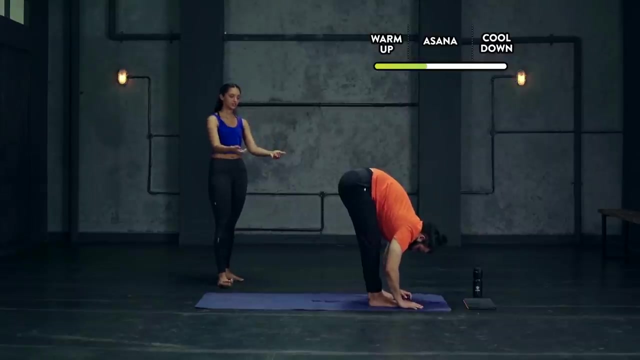 Once you're here, you're going to jump forward with the legs between the palms- Padangushthasana. Now keep your feet a little apart here, Create a little bit of distance about hip width, And now you're going to bend forward completely from the hips, bringing the palms and using 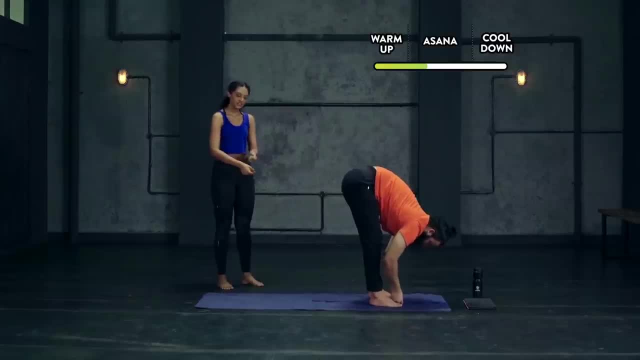 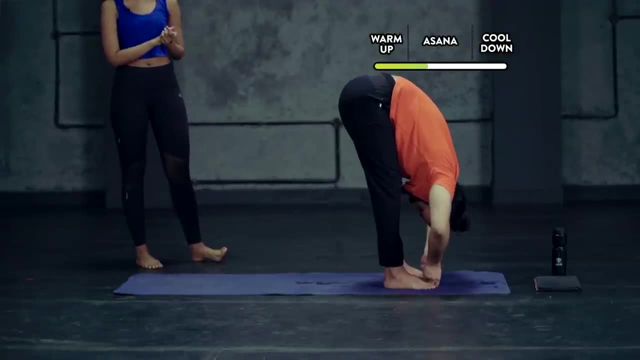 the fingers to catch your big toe. Once you've done that, really bend forward as much as you can, bending the elbows softly. If this is challenging, keep the knees softly bent. We're going to hold for five breaths And then we're going to release the palms And 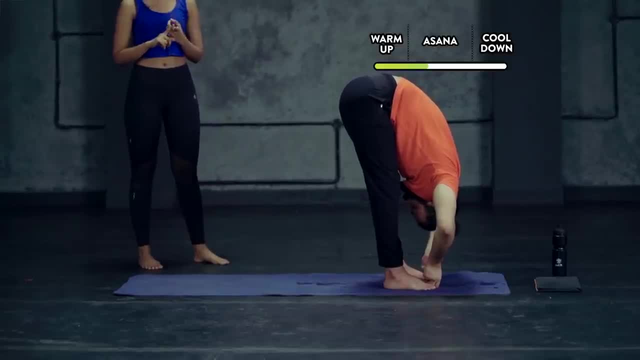 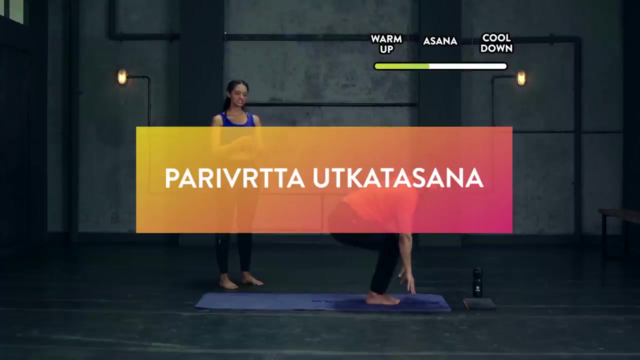 we're going to hold this now over here for five counts: One, two, three, four and five. Second asana. we're going to come into Parivritta Utkatasana, Legs together now, Bending the knees and sinking the hips down. Now bring the hands into a Namaste at the chest and 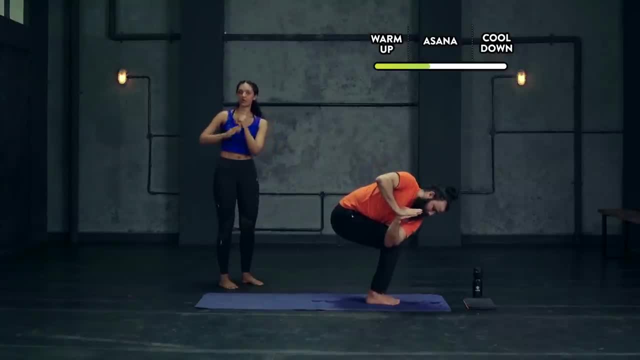 start to twist your spine completely, Left elbow outside the right outer thigh Twist in such a way that your toes are not touching the ground, And then you're going to come into Parivritta, Uttara T frost. So for this asana, try to bring your right foot up a little. bit more, push your legs a little bit more out, and then you're going to pull the right leg. So let's do it for five breaths, And this time I'm going to bring the left hand to your chest And then again you're going to pull the left hand back, step your left. 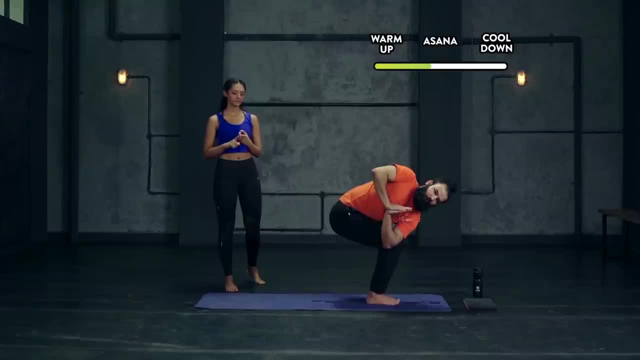 foot to the left and now grab the right leg, Bring the right leg back, stay there for 5 breaths. We're going to hold this now for five breaths: One, two stay there Three, four and five. 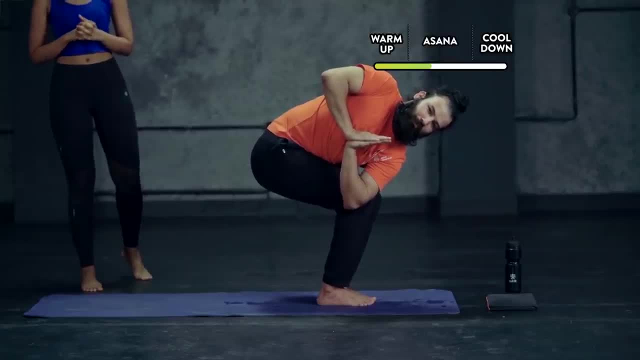 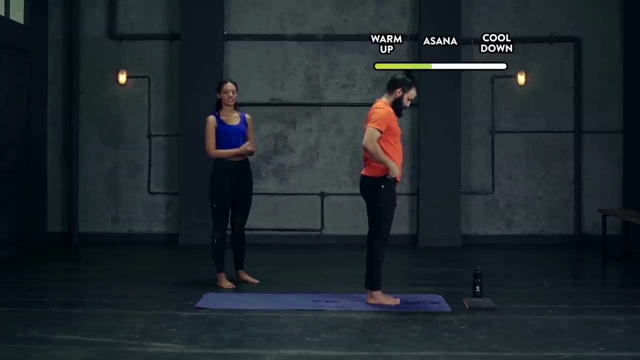 Now transition. Bring the Namaste back in the front of the chest, Come into a simple Samastitih position. The third asana from here is Parivritta Trikonasana. So step the left leg back, creating a mid-stance. 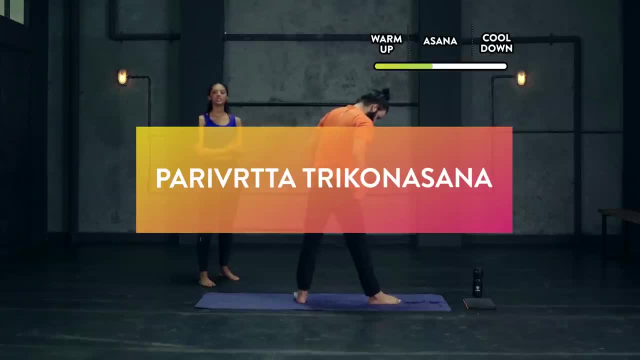 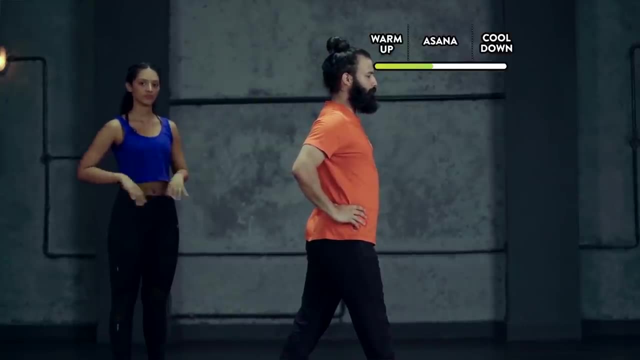 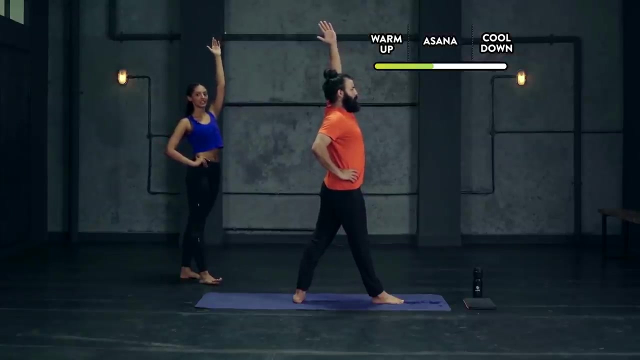 between your legs, the left leg back, creating a mid stance between your legs and making sure the hips and shoulders and one line pointing in the frontal direction. hands on the hips. now take the left hand up, inhale, stretch it over the top, arch back slightly to get an extra stretch. now exhale and bend forward as. 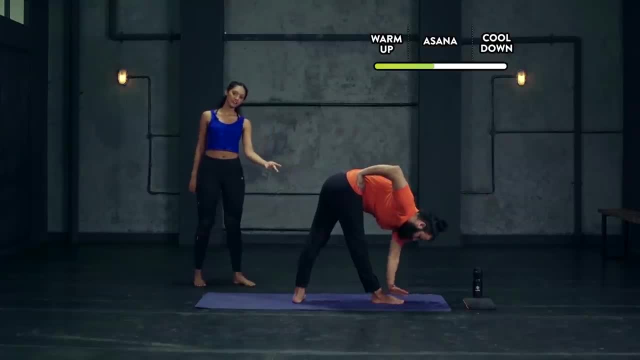 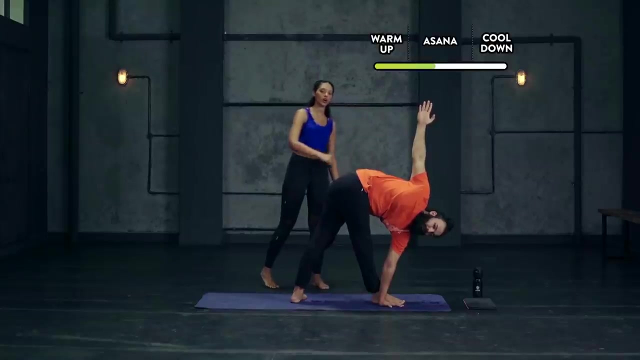 you do so, twist and bring your left palm outside the right foot. once you're comfortable, raise the right hand off the hips, completely straightening it, and stay in this position. make sure that you have a straight angle between your arms and now release, once you've stayed for a few breaths. 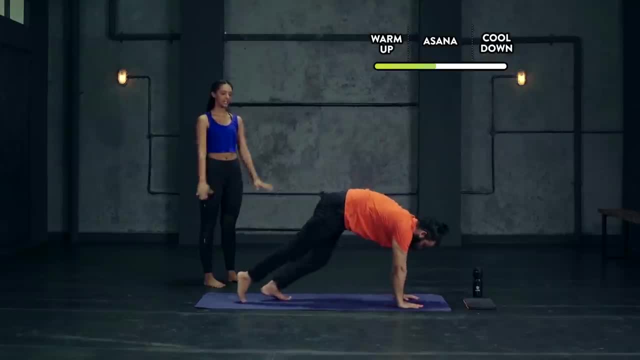 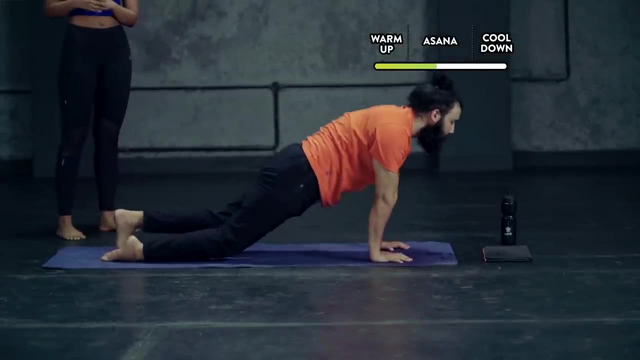 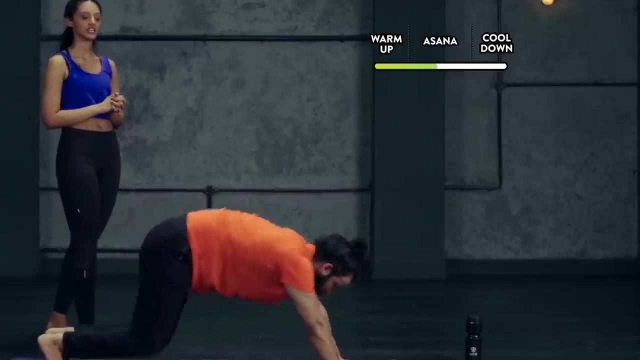 and come back, bring the palms onto the mat and coming into vinyasa. so chaturanga urdhva mukha, adho mukha. and we'll repeat the sequence right on the other side. So now jump forward, Badangushthasana with the legs between the palms. and now you're. 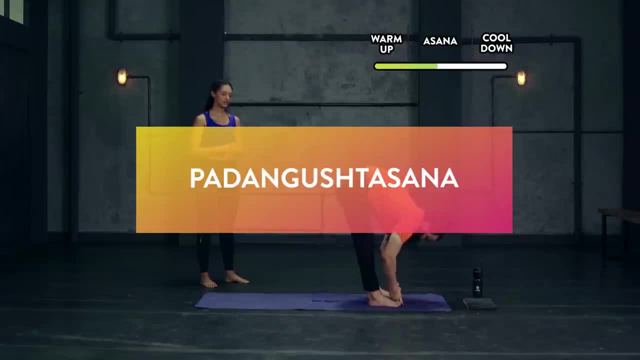 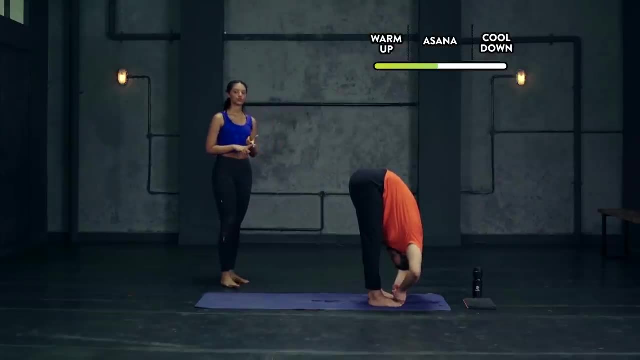 going to bring your hands towards the toes, completely bending forward, and leave the elbows relaxed. one, two, three, four and five. Now coming up legs together: Parivritta Utkatasana, on the left side, taking the Namaste at the chest, placing the right arm outside the left thigh. 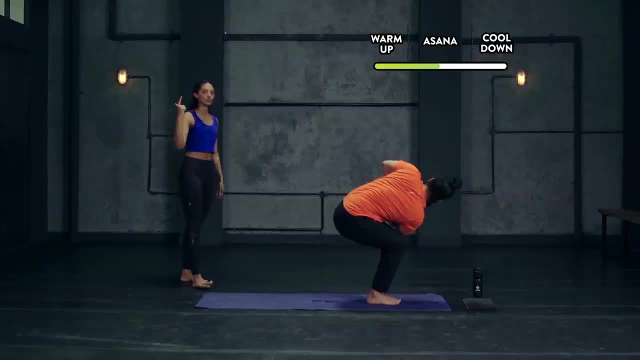 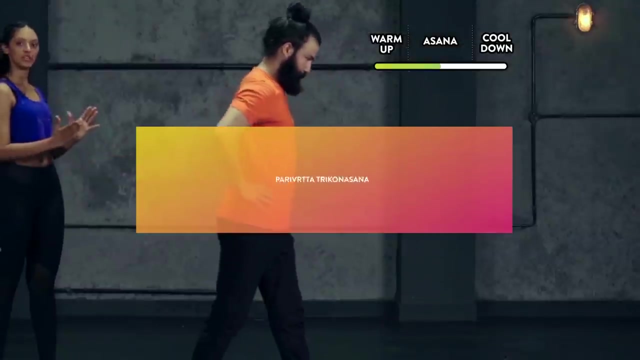 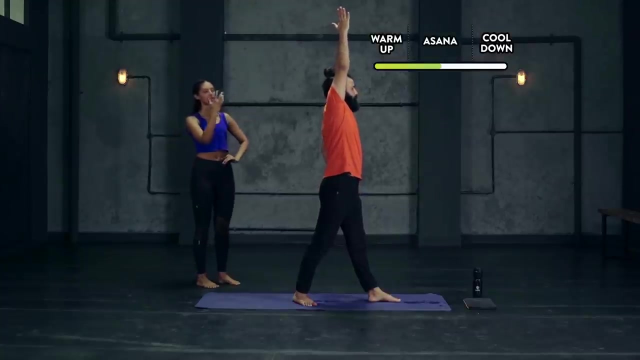 opening out the chest completely. one, two, three, four and five release Parivritta Utkatasana. come into simple Samasthiti. now bring the right leg back, mid stance. make sure the hips and shoulders are in one straight line. hands on the hips. take the right arm up in line with the ears. inhale arch. 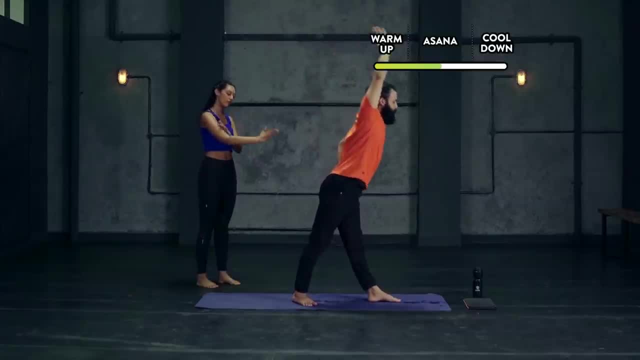 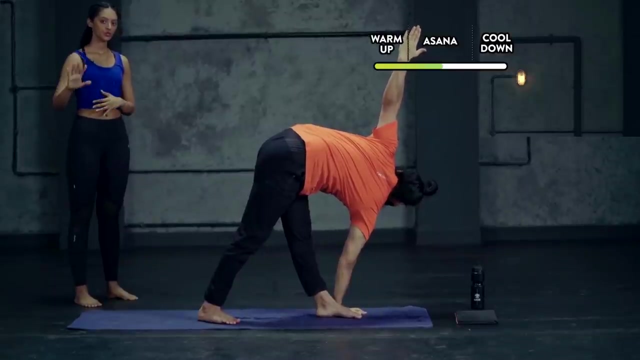 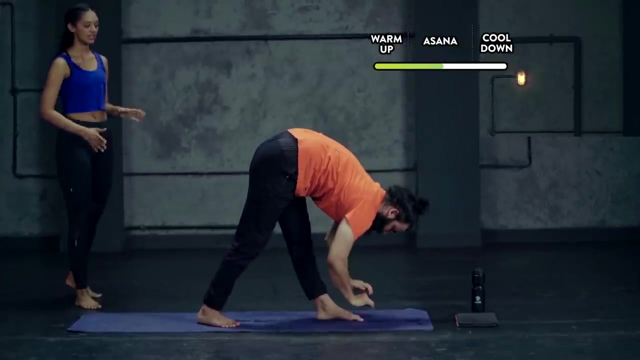 back, exhale and bend forward completely, taking your right palm outside the left foot. once you're comfortable, open and extend the arm completely, staying here for five breaths: one, two, three, four and five. release the twist, bring the hands back, placing them on the mat and moving swiftly. 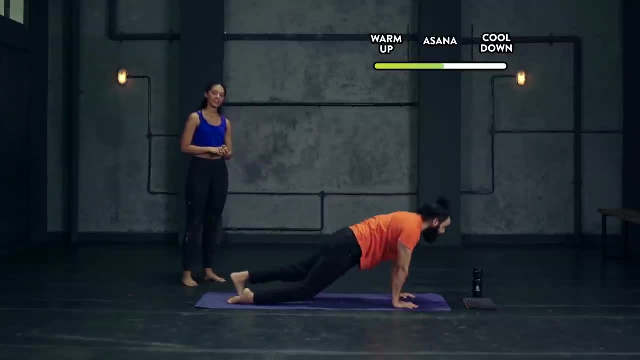 Urdhva Mukha, Adho Mukha and release. fantastic. now drop the knees down and rest in child's pose. that was our second sequence. i hope that you're feeling energized and you're really feeling the essence of power yoga. we're now going to begin with our third sequence. 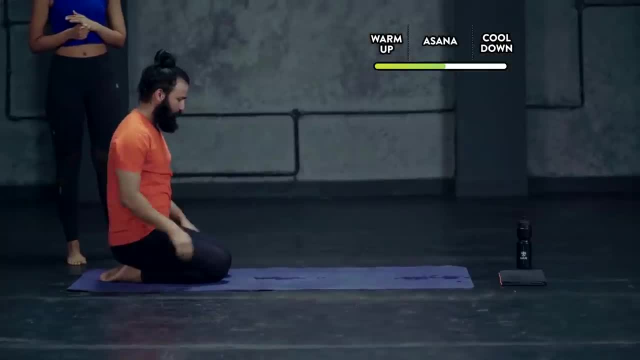 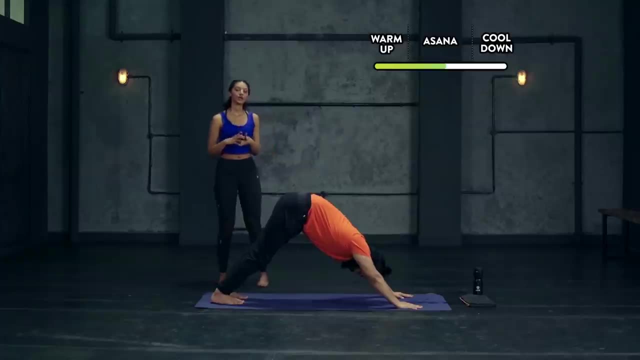 so let's learn how to practice this. coming into your simple Adho Mukha Svanasana, tuck the toes in hips rising upwards. so now we're going to start with Ekapada Adho Mukha Svanasana, so take the right leg up, raising it. 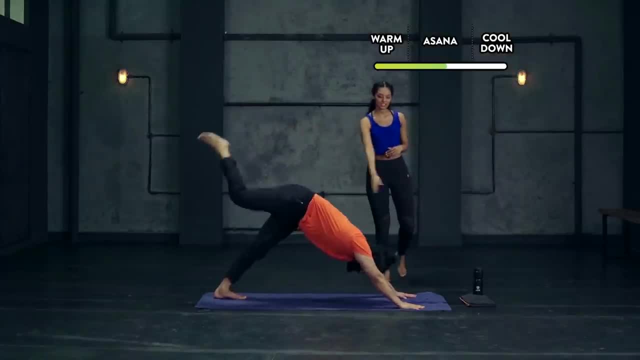 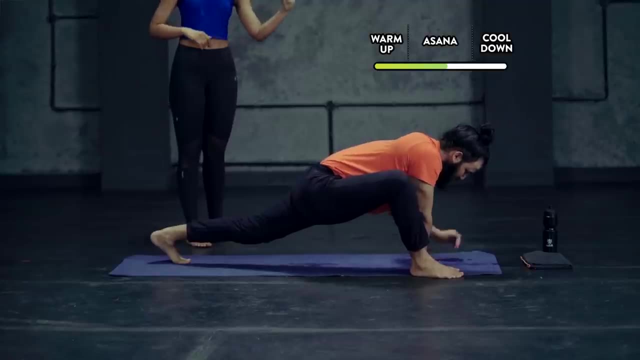 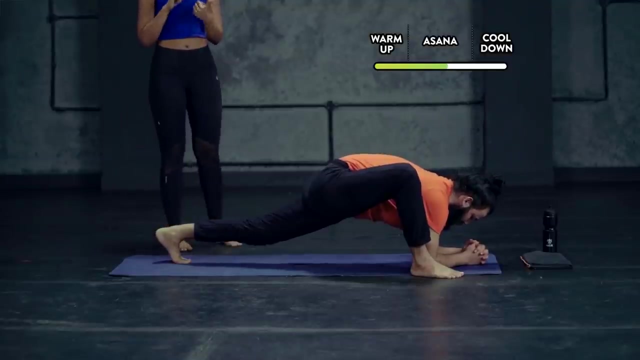 all the way to the top. now swing the right leg and bring it down outside the right palm. this is Uttana Prishtasana, left knee off the mat. slowly start to place one elbow at a time. interlock your fingers and hold this position for five. one, two, three, four and release. 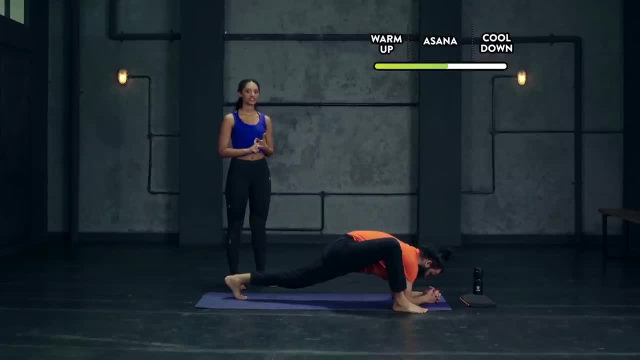 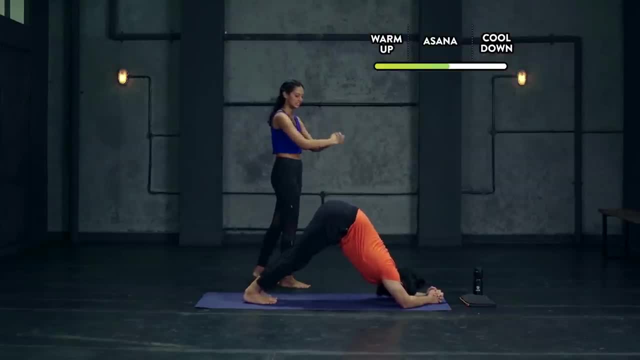 heels flat on the mat. remember, your hands are still interlocked. now let's begin the first rep, taking the chin forward, extending, trying to bring the chin to the mat and then coming all the way back with the hips rising upwards. we'll repeat this now four more. 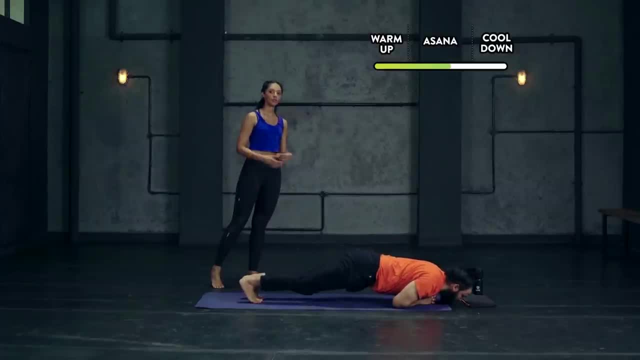 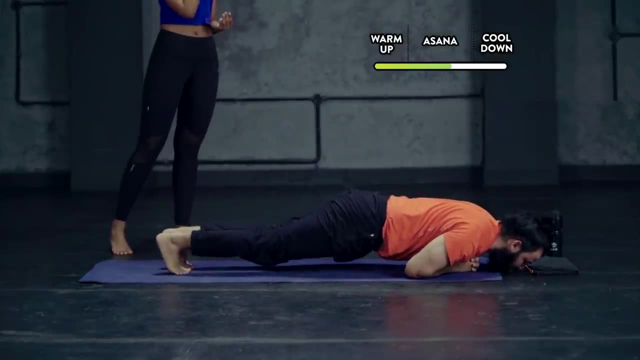 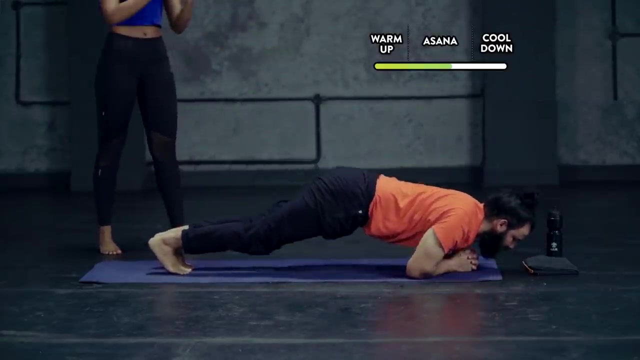 times come forward with the chin, placing it on the mat and back into the pose. third one, all the way down, placing the chin to the mat and back. fourth, going forward- you've got this slowly coming back- and the last rep, fifth, all the way forward: chin to the mat and 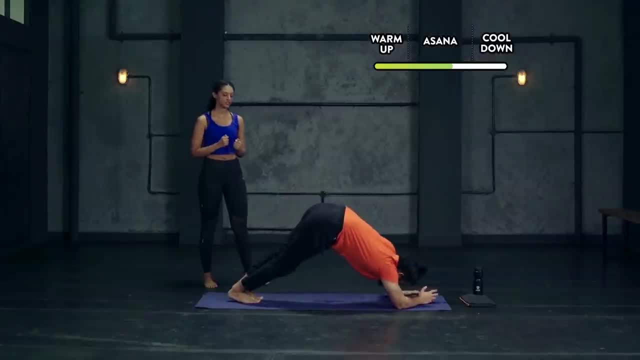 slowly coming back. now, release your hands. let's go into a vinyasa. so chaturanga urdhva mukha, adho mukha, all the way back. and now our third posture is going to be bakasana. so for this, you're going to jump into malasana with the legs outside the palms. from here, let's. 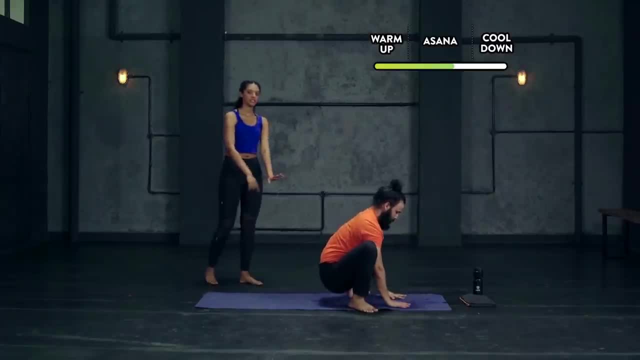 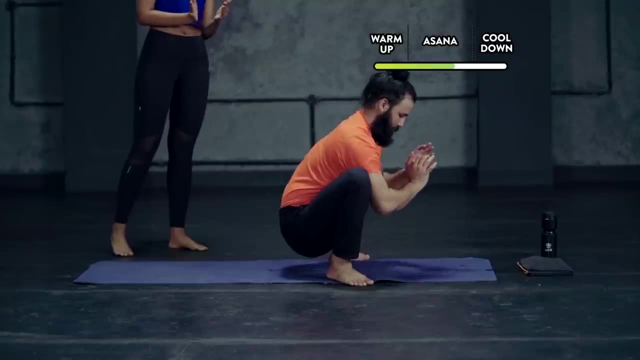 learn bakasana placing the palms on the mat, making sure the wrists and shoulders are in one line. you're going to start to transition, shifting your weight onto your hands as much as you can, make sure the thighs are pushed out now as you transition and shift your weight. 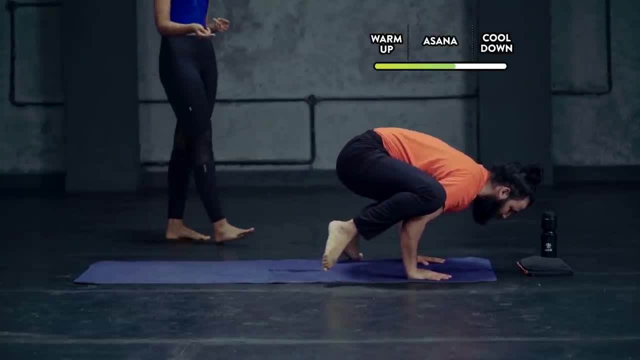 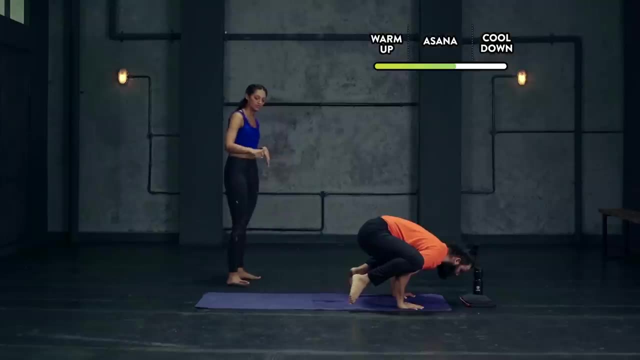 onto the hands slowly and gently. your legs will come off the mat when you're ready. right, you're balancing entirely on your wrists. look forward, chest open, hold for five. one, two, three, four and five. slowly start to bring both the feet on the mat. bring the hands back, placing the palms gently. 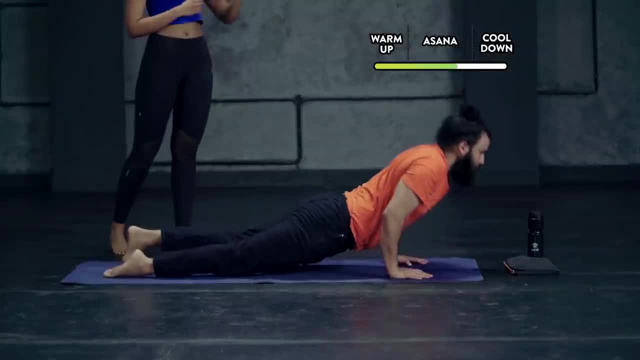 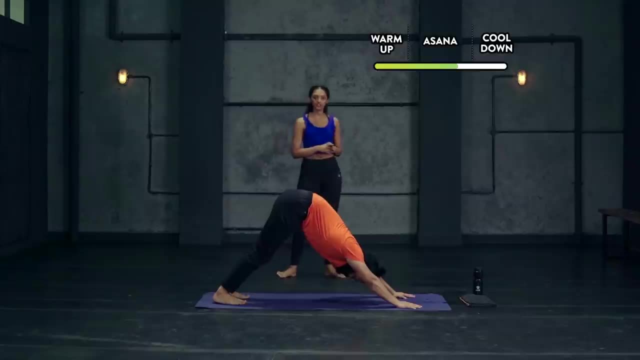 on the mat chaturanga, urdhva mukha and adho mukha once again. right now, let us repeat the same sequence on the left side, taking the left leg all the way to the top. now swing, bring the left leg back outside, outside the left palm. 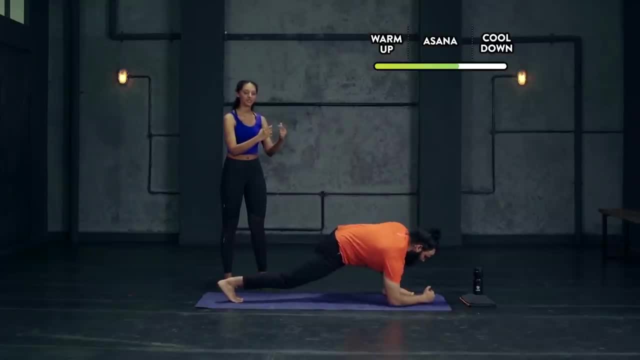 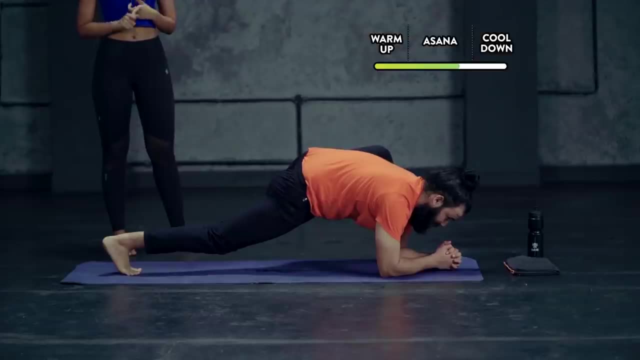 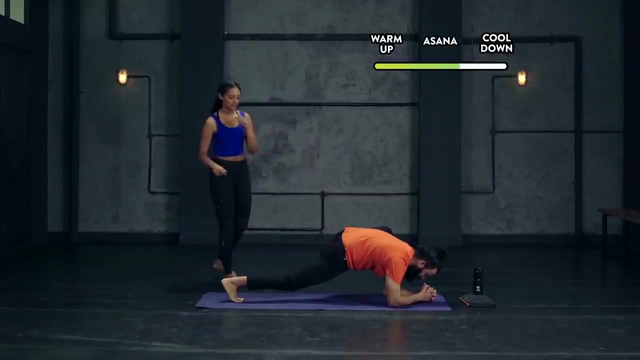 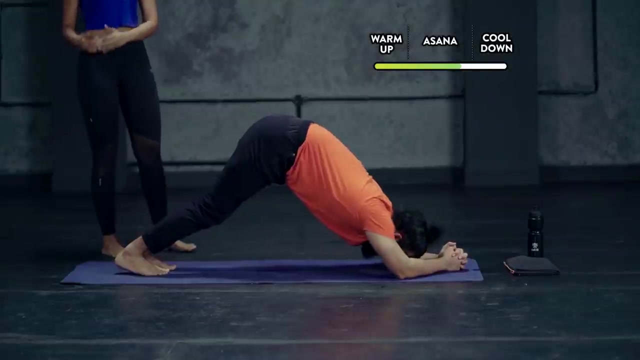 make sure the right knees off the mat, dropping the elbows down. interlock the fingers and hold one, two, three, four and five. now bring the left leg back to the right leg. dolphin push-ups. now, hands interlocked, begin, take the chest and chin forward, placing it on the mat, and slowly rise up. come back second rep all the way in the front, chin to the mat. 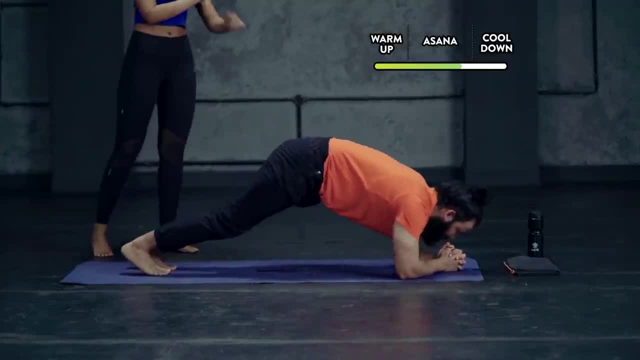 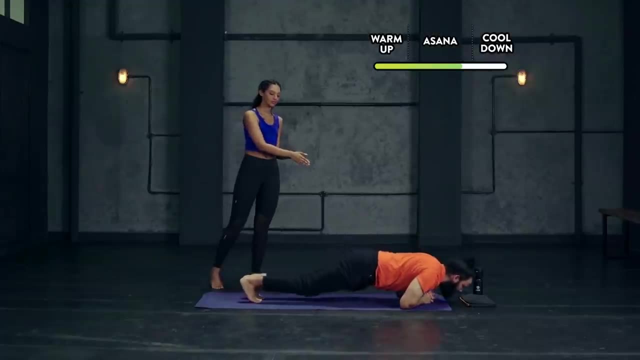 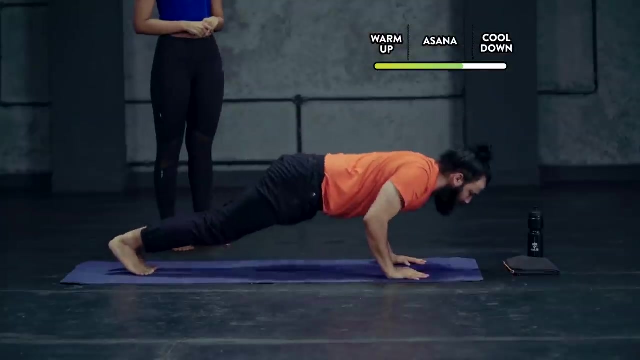 and back. third rep, moving forward, keeping the pressure on your arms and shoulders, and back forth. rep, moving to the bottom, all the way down and back. last one, moving the chest and chin all the way to the ground and coming back up. fantastic, now release the hands. quick vinyasa here, chaturanga. 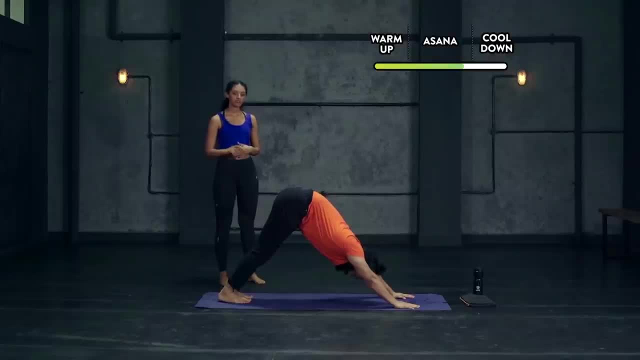 exhale and adho mokha. brilliant. now, from here, we are going to do bhakasana once again. so jump with into malasana, legs outside, placing the palms on the mat in a straight position and then starting to мужчi vatsana. 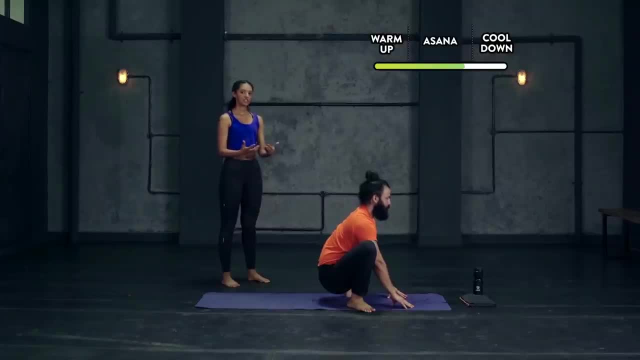 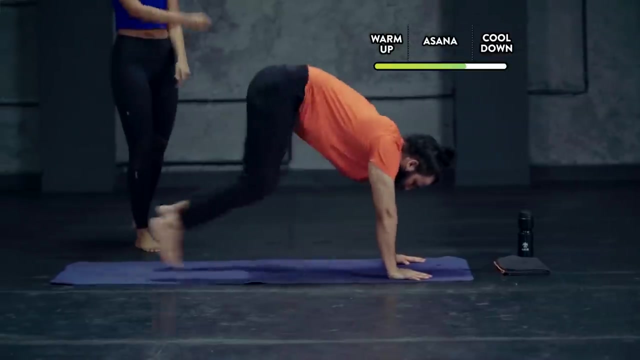 mat, making sure you've got a good grip. now transition: shift the weight forward completely onto the palms and come into bakasana with the legs off the mat. one, two, three, four and five release. bring the legs back quick. vinyasa over here. jump back into chaturanga. urdhva mukha inhale. 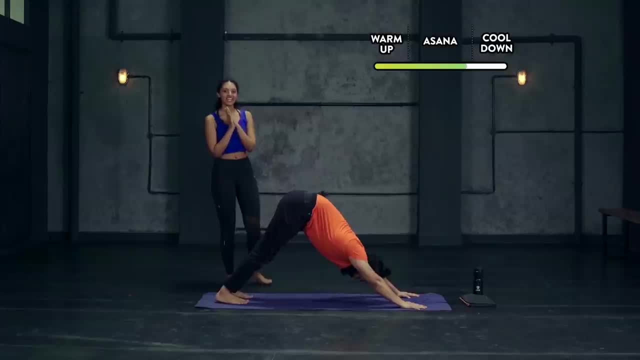 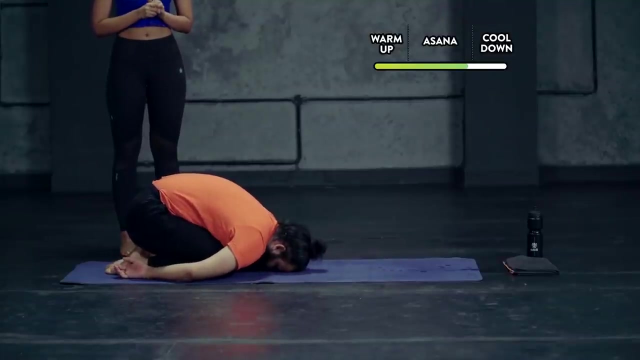 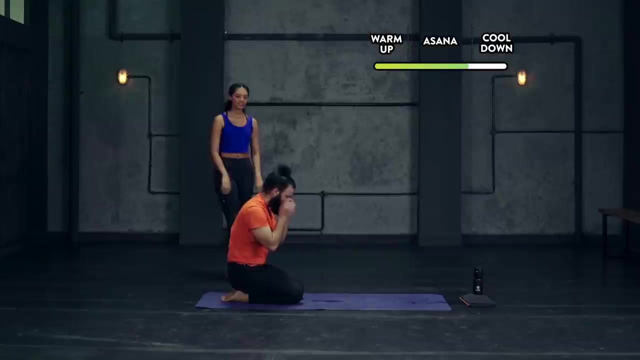 exhale and come back great stuff. that was the end of our third sequence. drop the knees down on the mat, relax in child's pose. stay here now for just three breaths: one, two and three. right fourth sequence, now coming once again into other mukhashvanasana. 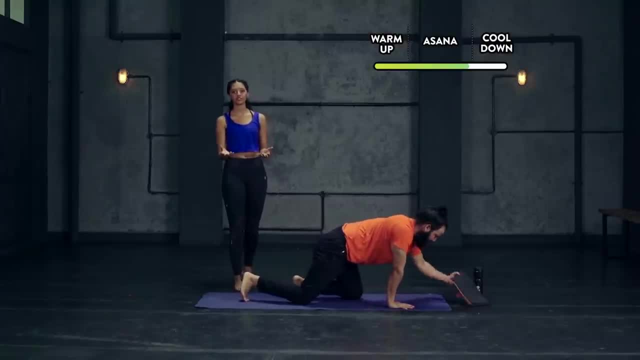 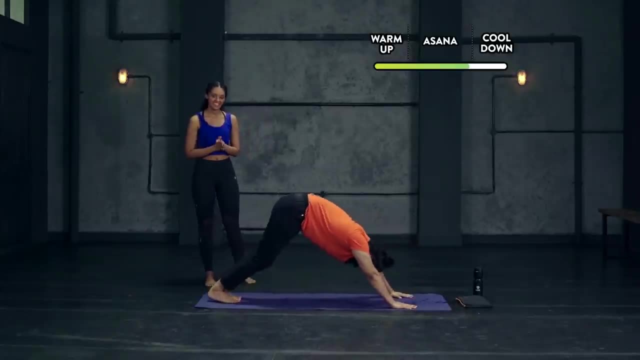 please feel free to wipe off your sweat. take a slight break if you need to. I understand this is quite a challenging practice, So please go at your own pace throughout this session. Let's begin sequence 4, Adho Mukha Svanasana. 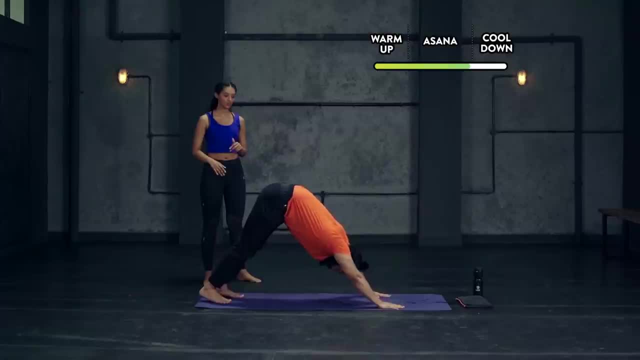 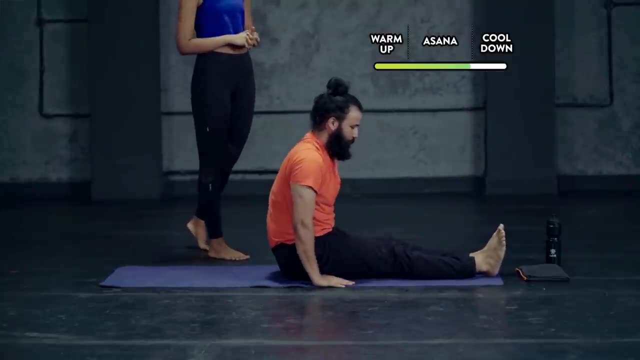 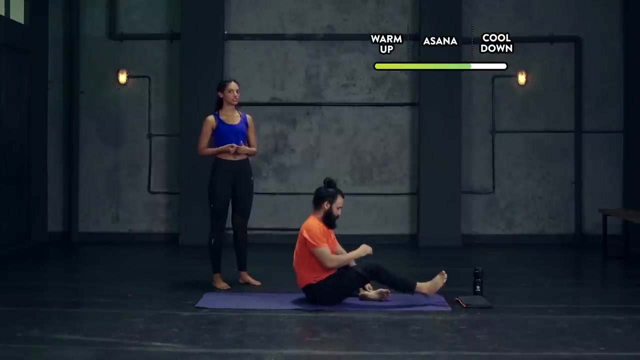 Now we're going to jump through and take the legs forward. Alright, so once you're ready jumping through and coming into a cross legged position, extending the legs forward, The first asana is Baddha Konasana, or the butterfly pose. So bring your legs closer to the perineum. 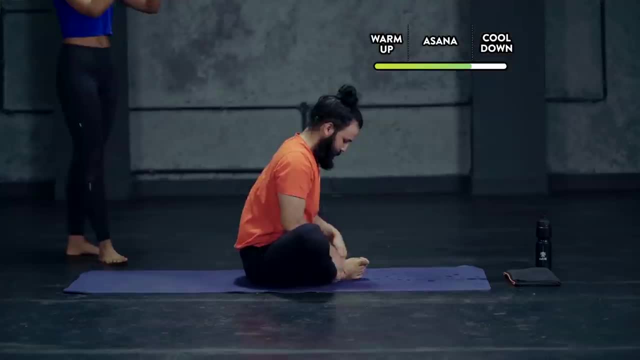 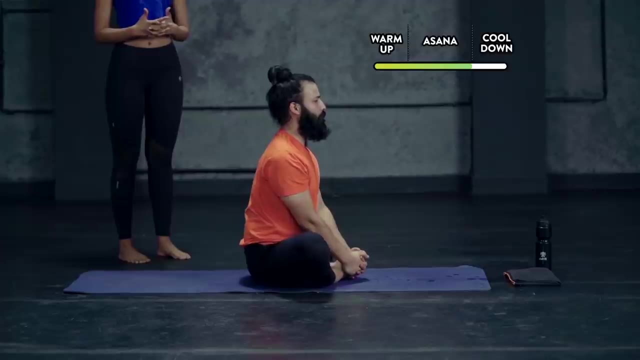 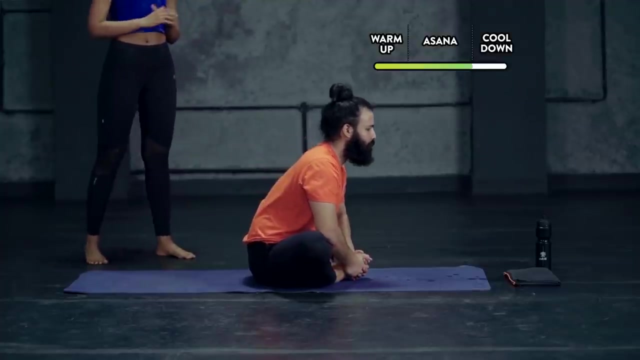 region, placing the feet together and now interlock the fingers, placing them underneath the feet. Roll the shoulders back, spine lengthened. Once you're ready, using the pressure of your hands, fold forward very gently and slowly, going as per your own capacity. Once you have. 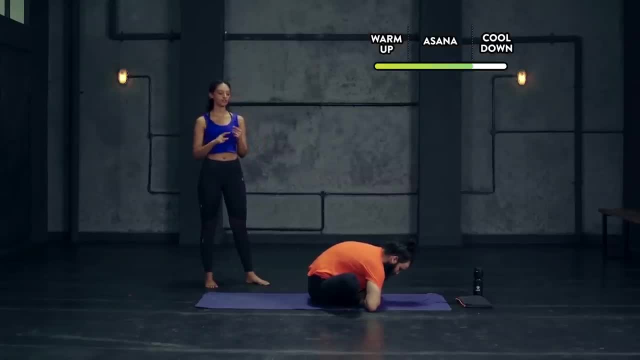 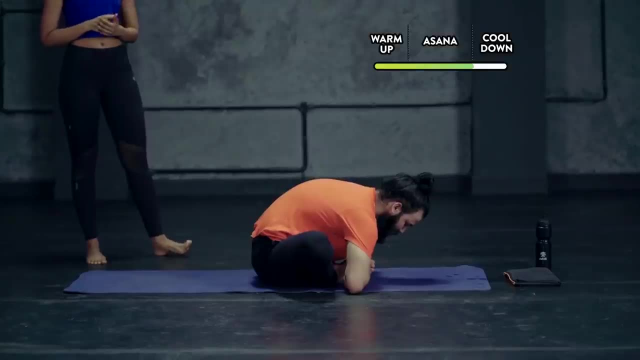 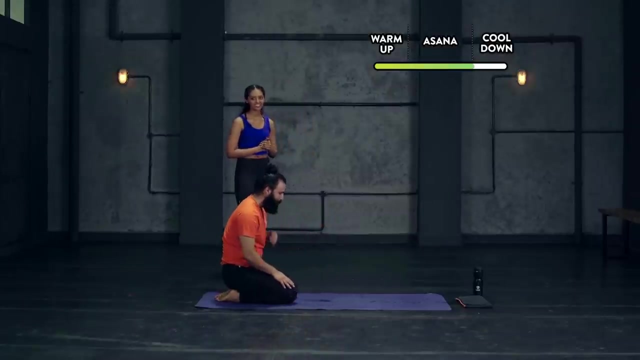 reached maximum capacity. you're ready to jump. Hold for 5,, 1,, 2,, 3,, 4 and 5.. Gently release your hands now. Now let's transition to our cooling down asanas. I'm sure this is quite a workout for all of you, but it's very important. 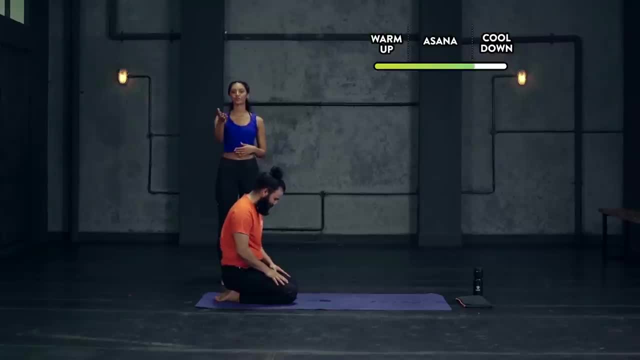 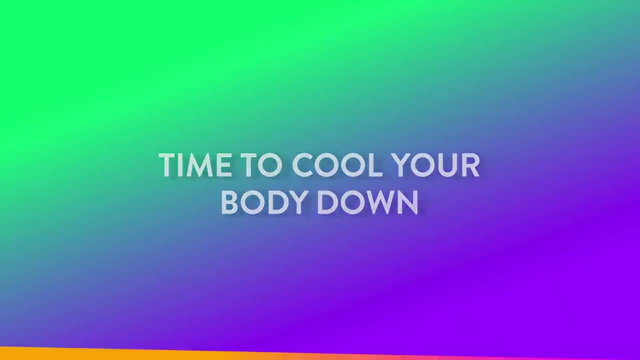 to cool down as well. So great job, Gaurav, and I'm sure you all did a fantastic job at home as well. Let's transition into the supine position now, So lying down on your spine, as you're comfortable Placing the head on the mat. just coming into. 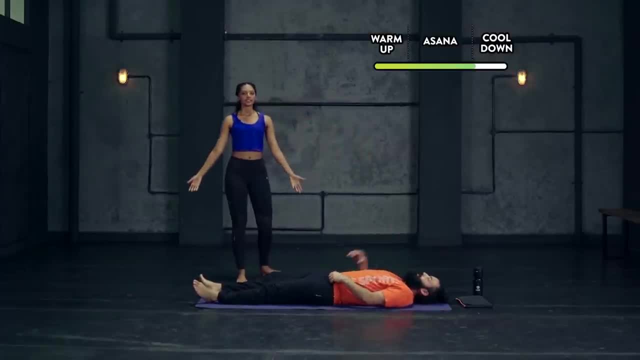 a simple lying down position And again, we'll just take two breaths here. Make sure you're comfortable, Wipe off any sweat that you have, And the first asana in the cool down position is going to be Chakrasana. So let's learn how to practice this You're going to bring. 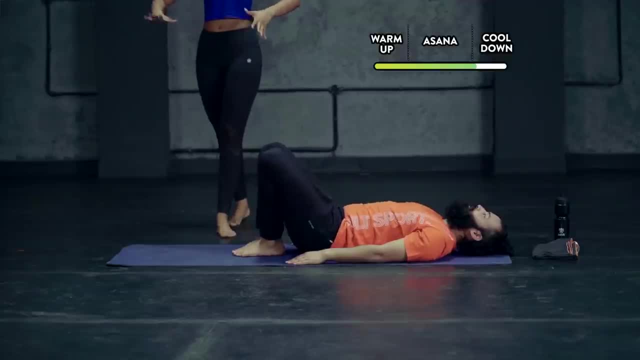 the legs together and fold them Now take the hands and place them close to your shoulders. So the next thing we're going to do is we're going to do a Chakrasana. So you're going to bring the legs together and fold them Now take the hands and place them close to 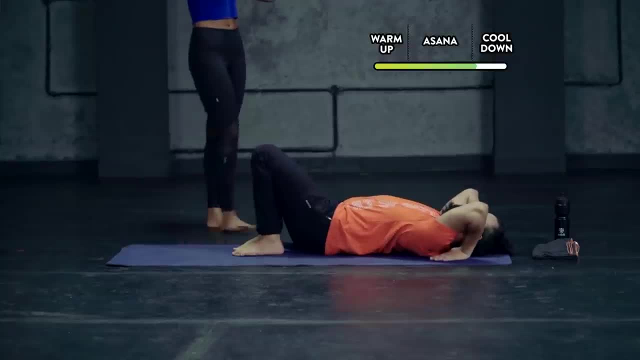 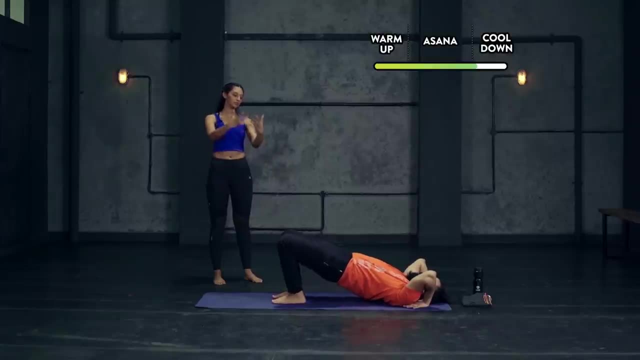 your shoulders. Now you're going to do a Chakrasana. So you're going to do a Chakrasana. Try to do it in line with the ears. In line with the ears, fingers wide, so you get a better grip. And now, when you're ready, you're going to raise the buttocks and hips up completely. 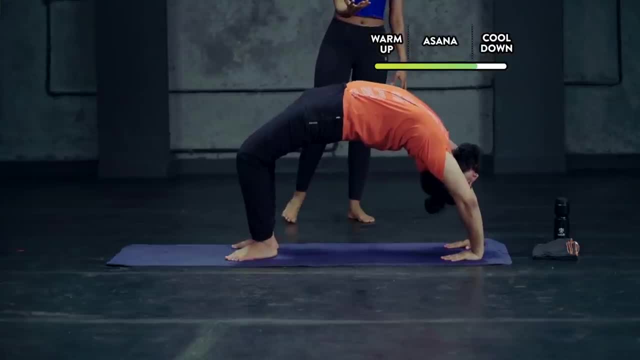 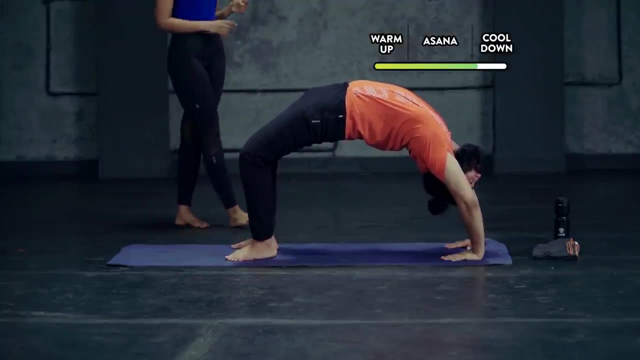 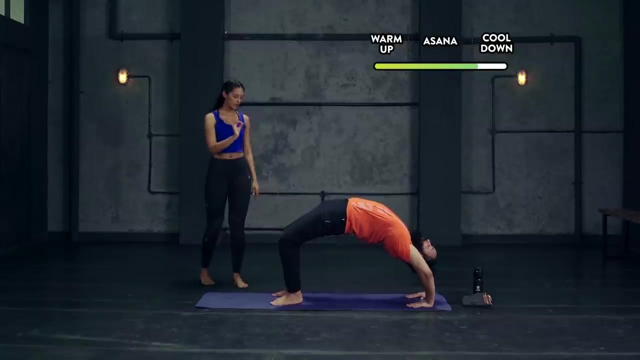 Coming into Chakrasana. As you rise up, try and hold this posture now for five breaths. Make sure you're feeling the arch and spine One, two, three, four and five Gently dropping down, Coming down. 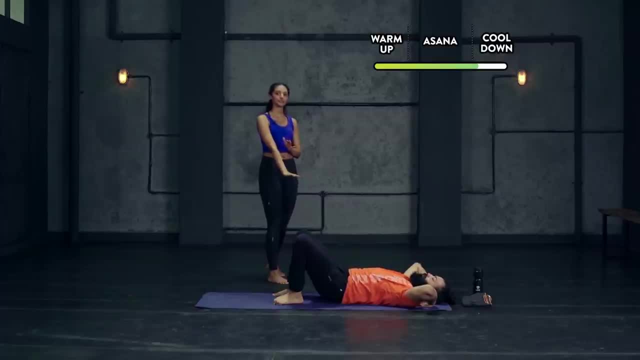 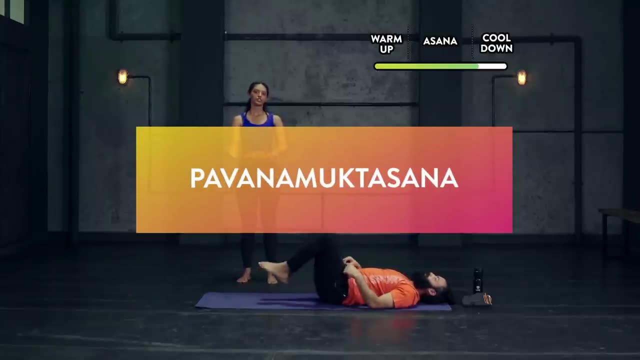 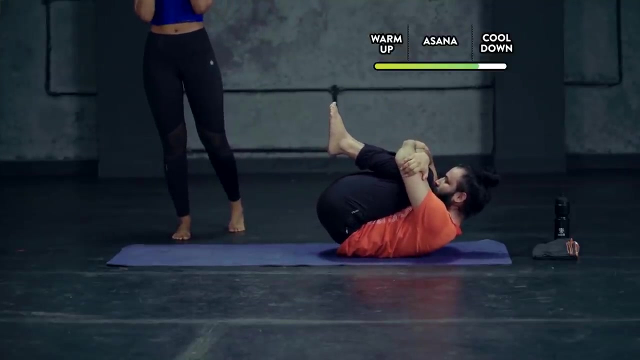 down with the head, shoulders first, then hips, and back on the mat. Release the hands and come into pavanmuktasana directly from here. So you're going to bring the knees close to the chest, hug them inwards and stay in this position with the neck raised upwards. You. 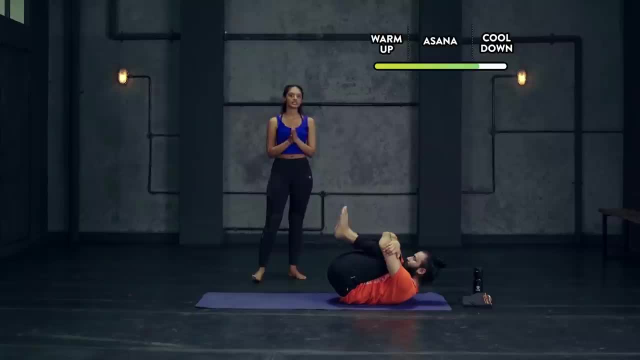 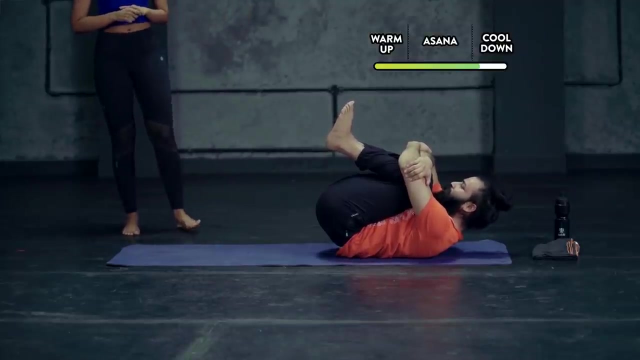 can either point the toes down or flex them in, whatever is a little more comfortable for you. Let's hold pavanmuktasana for 5 breaths: 1,, 2,, 3 and 4 and 5.. Now slowly release. 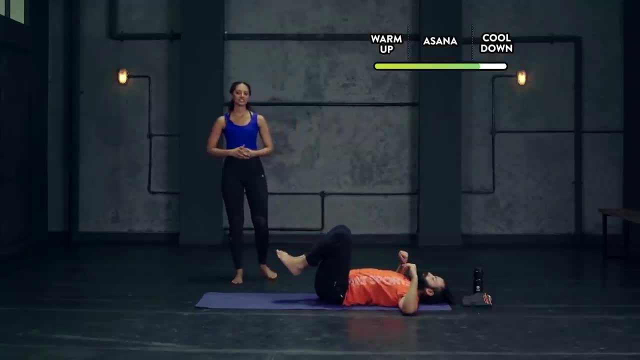 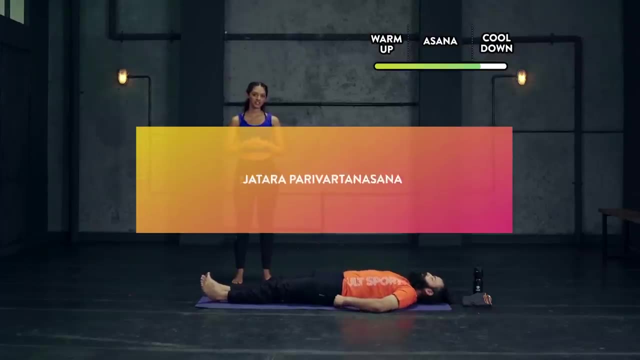 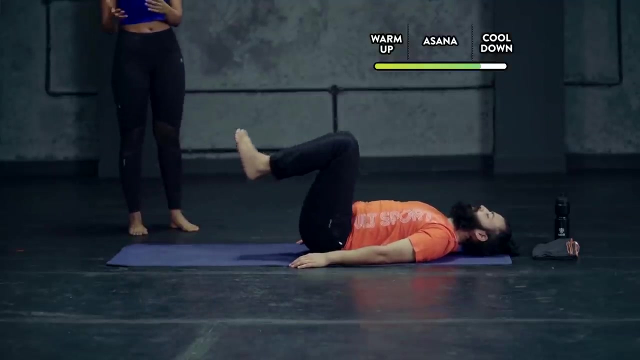 neck back, release the hands, release the legs and place them back on the mat. Now we have the final cool down asana, which is the jatara parivartasana. So let's learn how to practice this. Once again, you're going to bend your legs. this is a spinal twist, So once you've bent, 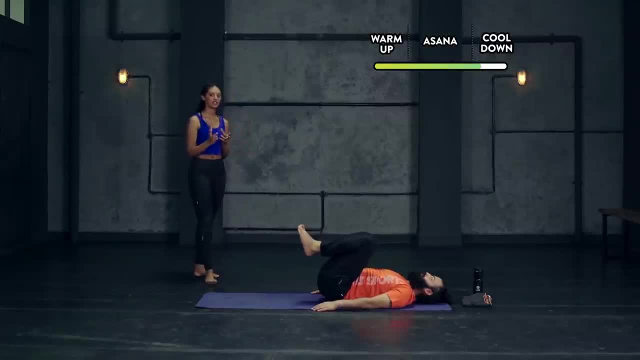 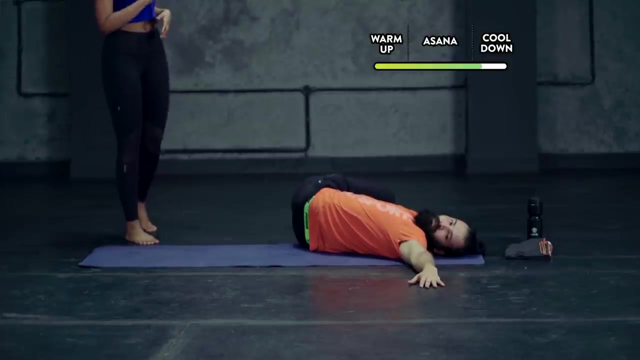 your legs. you're now going to slowly twist the legs towards the right side, bringing the arms up in the process and twisting completely to the right. As you do so, twist your neck to the left, feeling that spinal twist in this position. Let's hold here for 5 breaths. 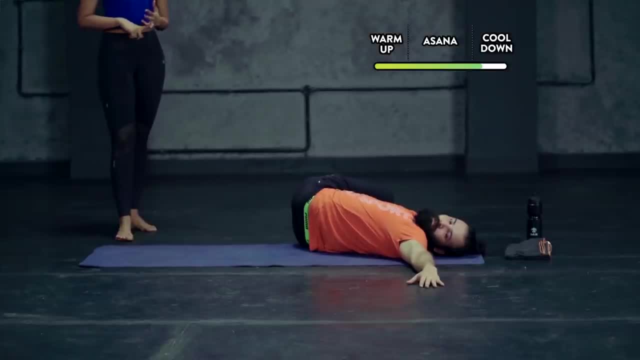 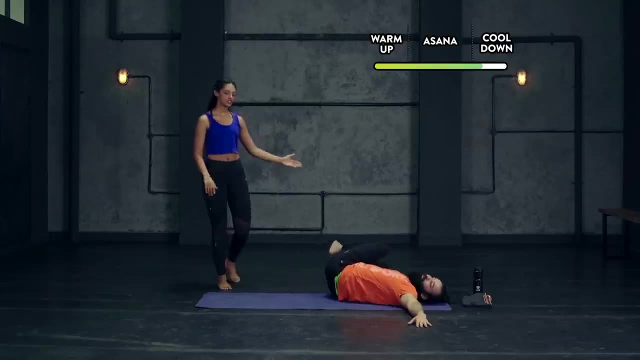 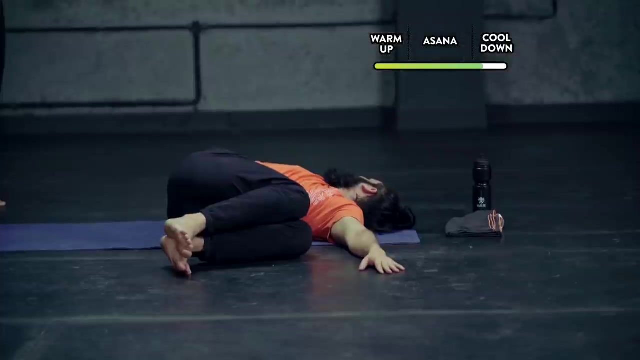 1,, 2,, 3,, 4 and 5.. Now smoothly transition leg back to the centre, head back to the centre, Take the legs towards the left. now twist completely and move the face towards the opposite side, Once again feeling that spinal twist, and hold for 5 breaths. 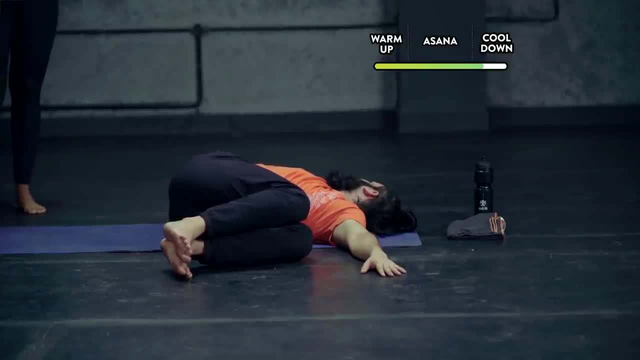 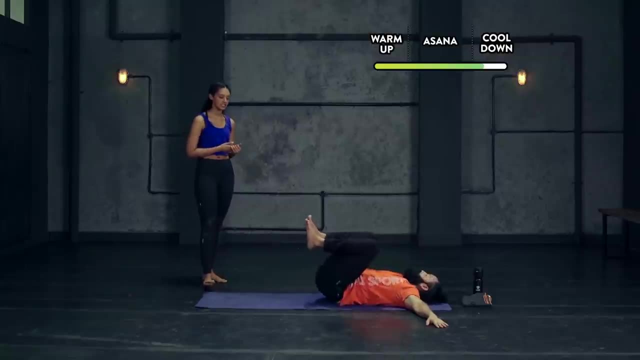 1,, 2,, 3,, 4, and 5.. now gently release, bring the legs back towards the center and release them completely. now on to the mat, bringing the hands back by the side of your body. now that we're done with our cool down asanas, we're going to transition into our 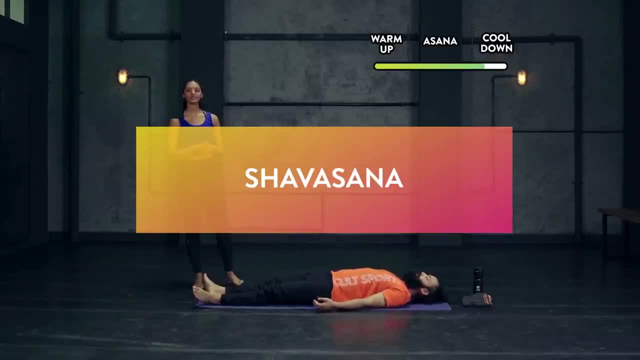 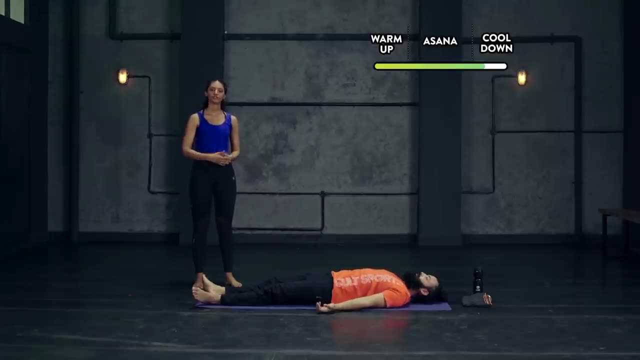 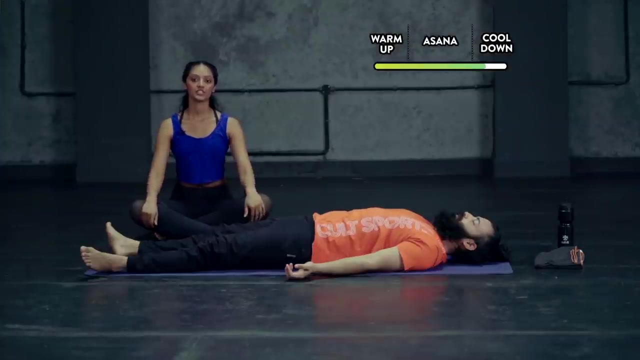 savasana. let's come into a very simple savasana position: palms facing upwards, fingers naturally curled a little bit of distance between your legs and head, neck and shoulders completely relaxed. now, as you come into your savasana, close your eyes gently and begin to focus all your attention completely on your body. 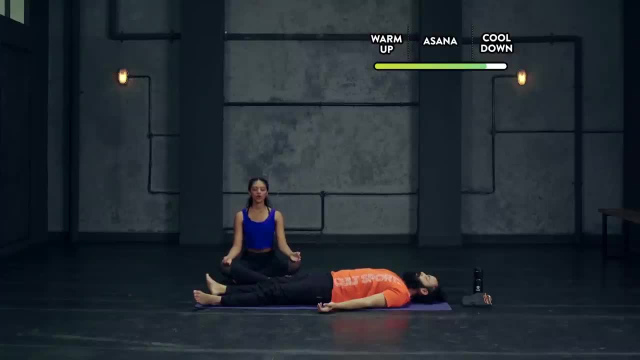 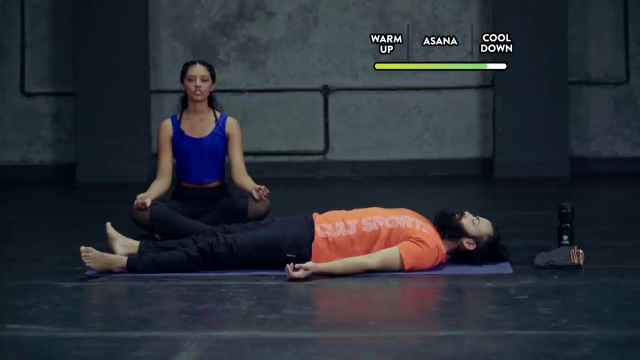 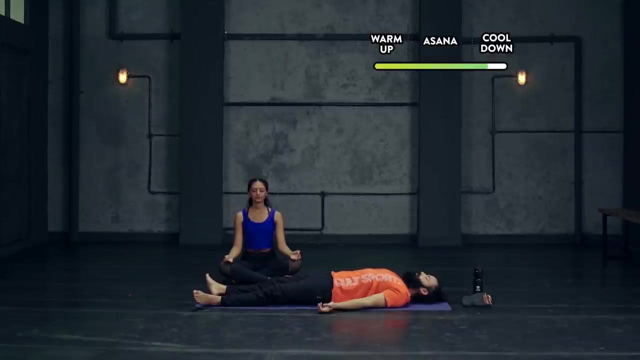 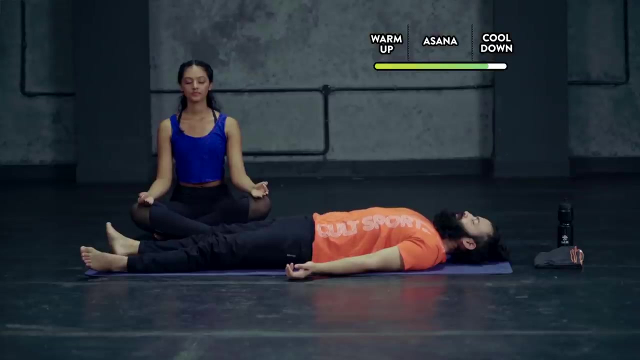 and now we're going to focus our attention completely on our body. focus all the way from the tips of the toes to the top of the head, relaxing and analyzing your body as we hold savasana in silence, now for a few minutes. stay for a moment and your welcom. there we go. 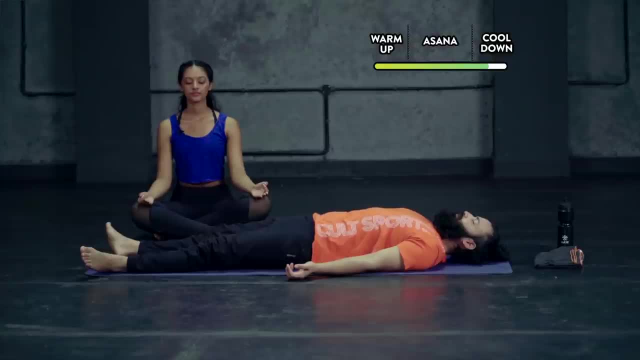 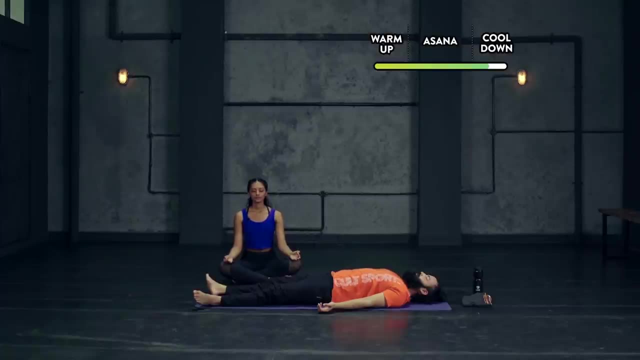 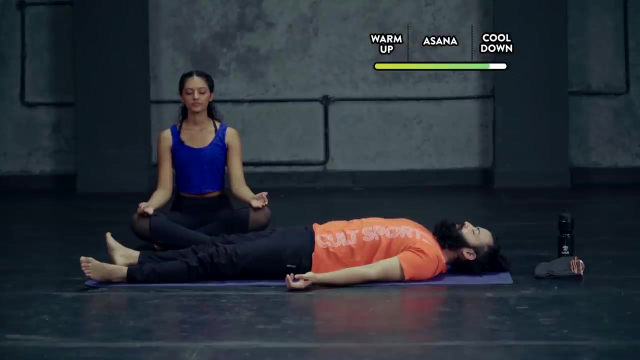 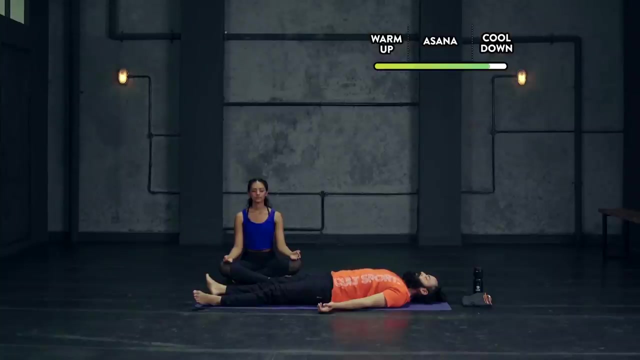 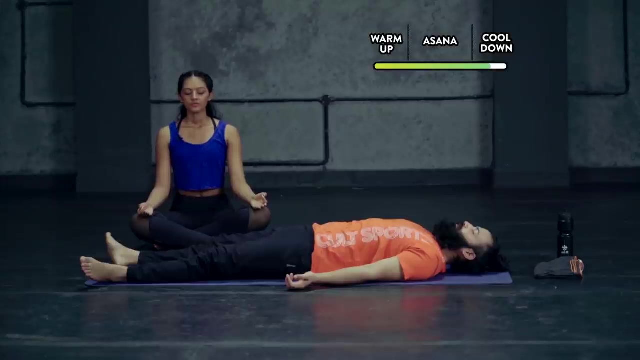 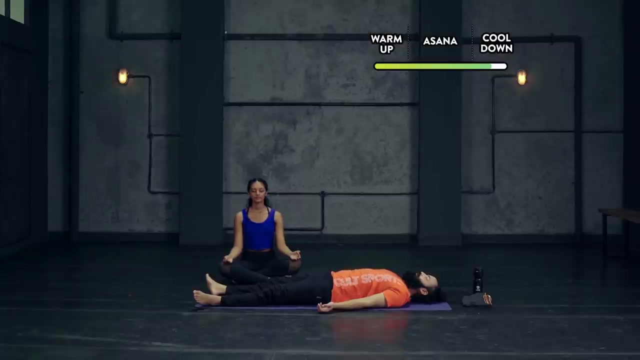 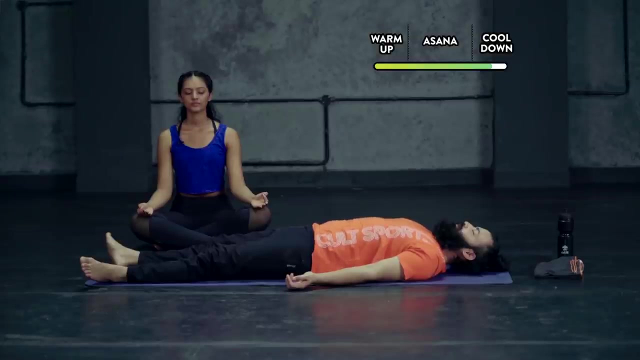 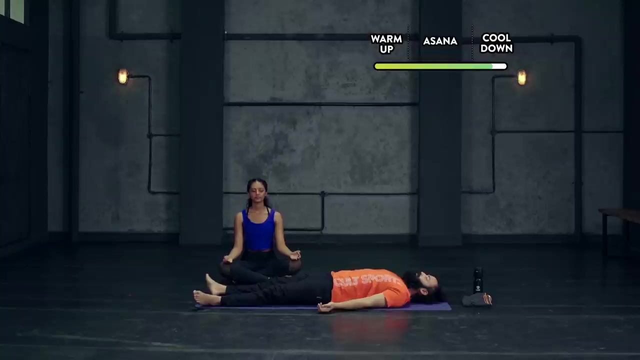 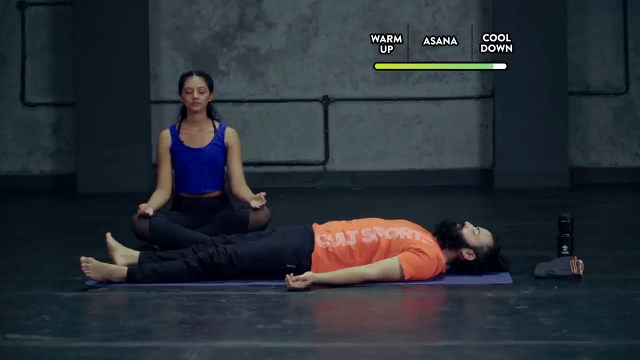 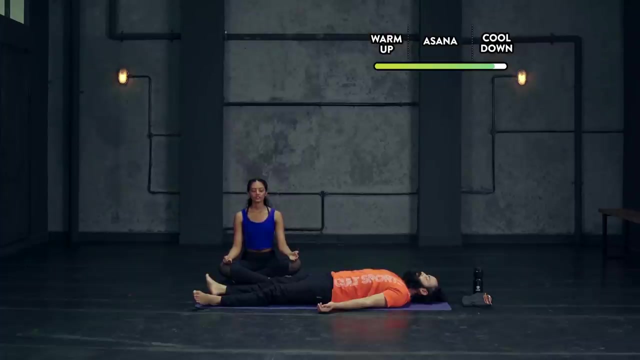 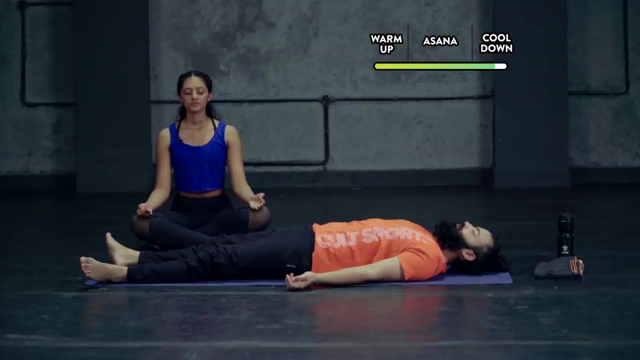 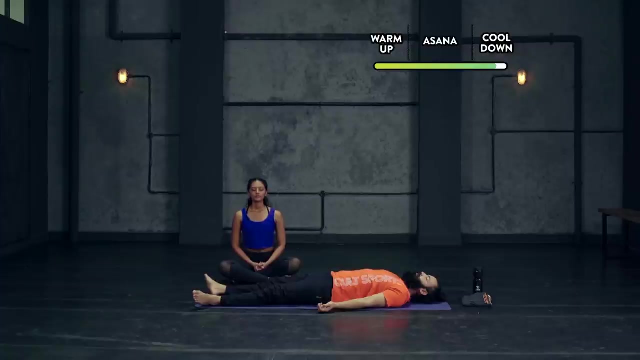 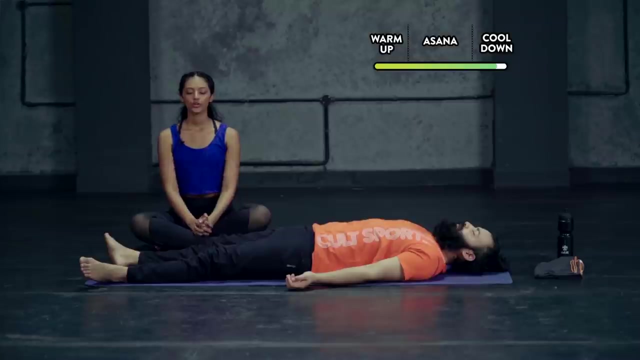 so that's all of this. so Thank you for watching. Thank you for watching. Thank you for watching And fully relax, Staying in this position For a few more seconds, And now slowly and gently start to bring your awareness back into the present moment. 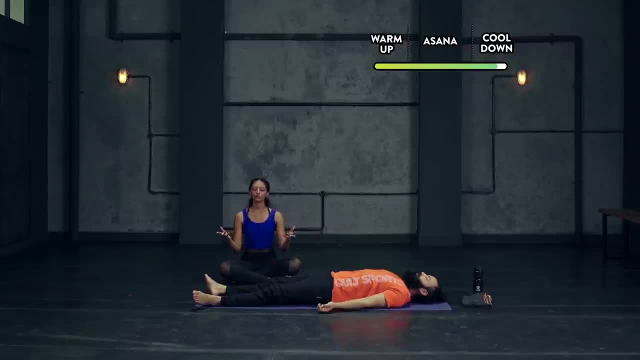 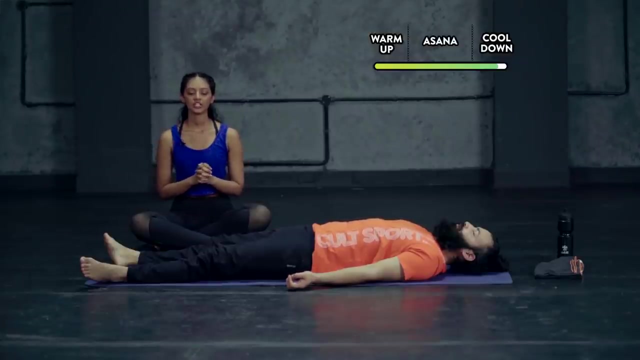 And as you do so, you can just move your fingers, move your feet just a little bit. to come back to the present, And now we are slowly and gently going to release our Shavasana. So now turn over onto one side. 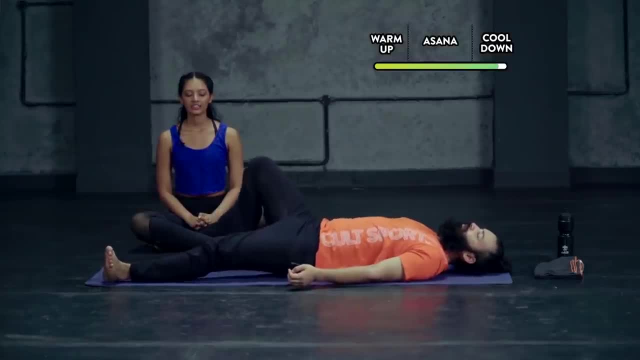 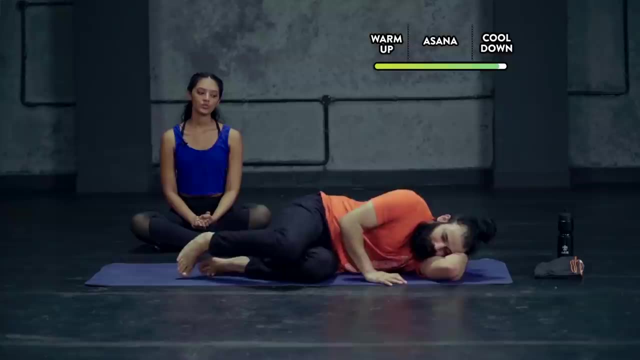 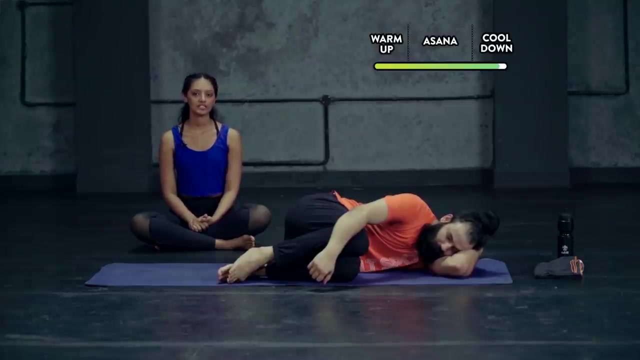 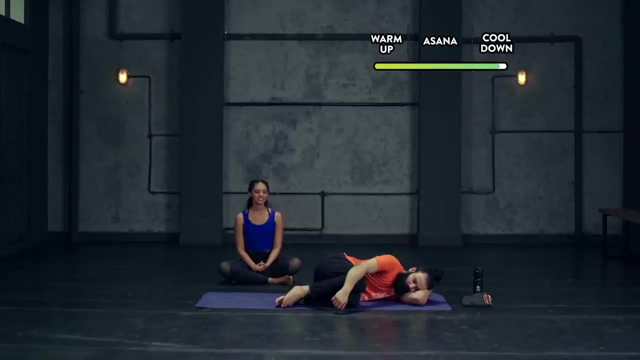 And as you do so, bring your hand underneath your head, Bring the knees in closer to the chest, Place the hand on the knees, Stay here for three long and deep breaths, Inhale And relax And exhale- Inhale- 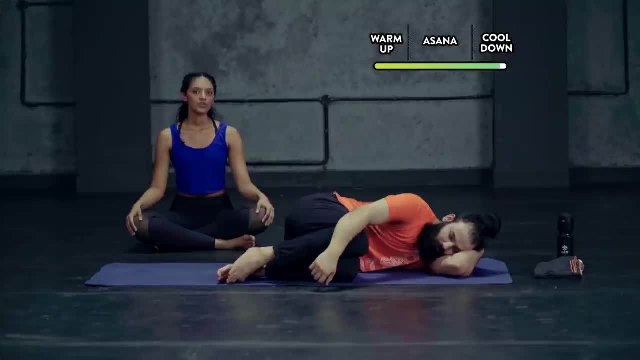 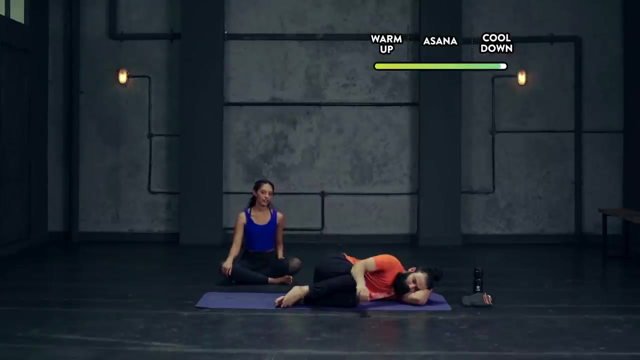 Inhale And exhale Again. Relax and exhale And Inhale one more time and Exhale Now. use the support of your hand to propel yourself into a sitting position as you come onto your mat. now Sit in Sukhasana, keep your eyes. 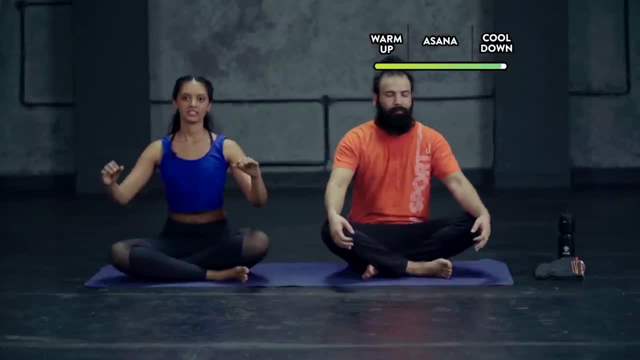 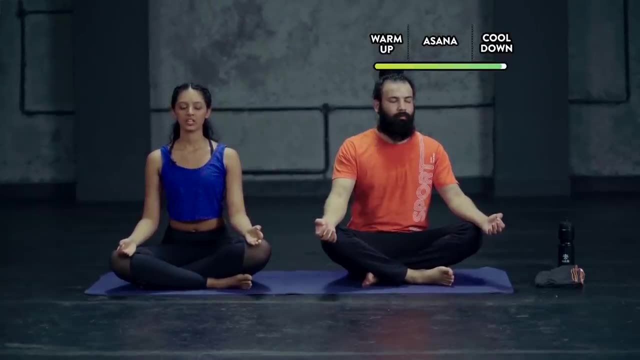 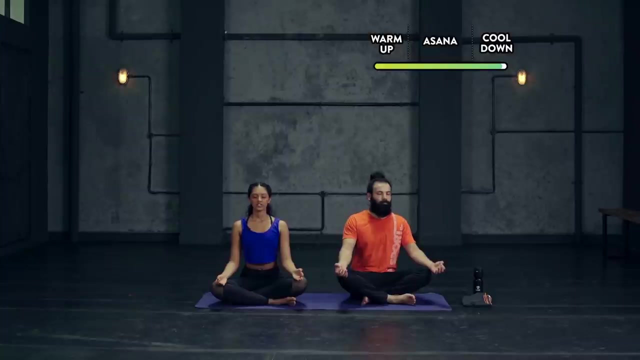 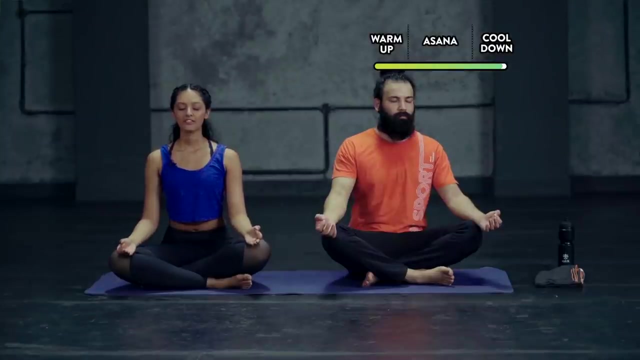 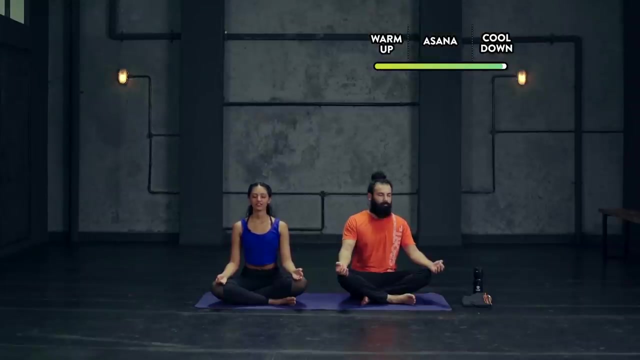 still closed. Bring your hands into Gyana position, place them at your knees, spine lengthened, chin parallel to the mat, shoulders rolled back, once again directing your attention to the breath. we have done an absolutely fantastic job today and we should be grateful and thankful for today's practice. 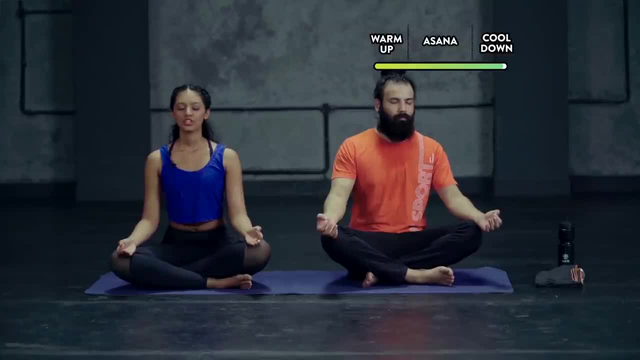 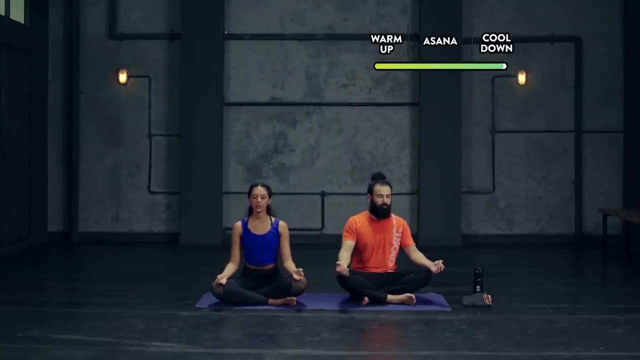 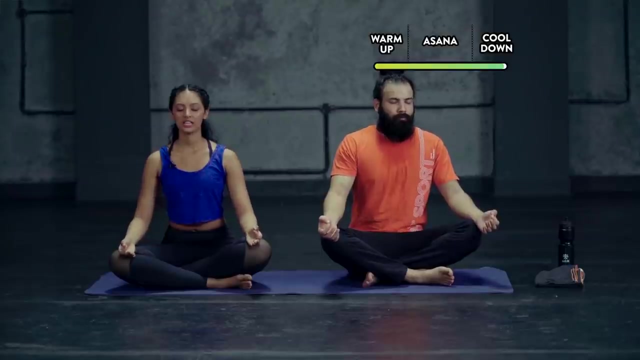 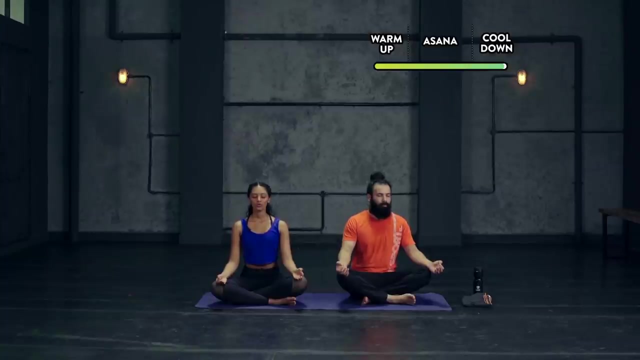 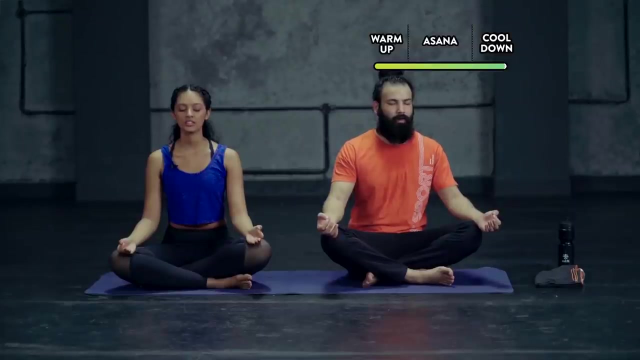 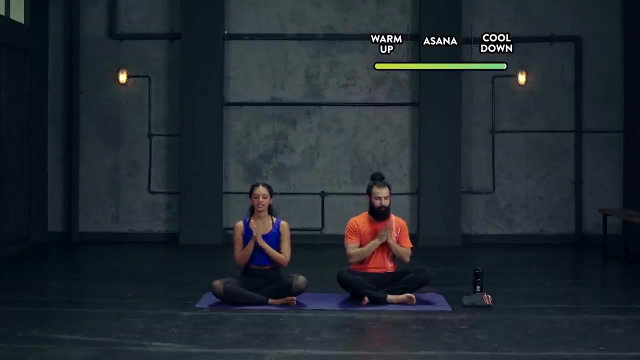 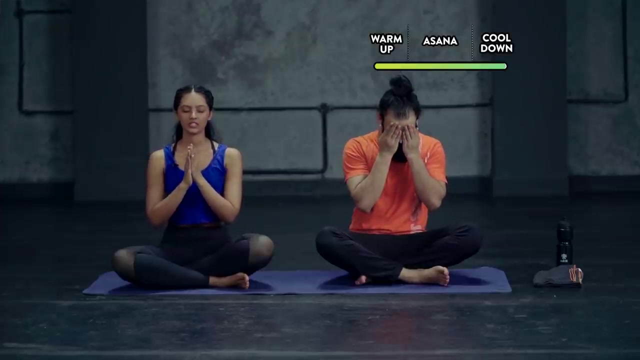 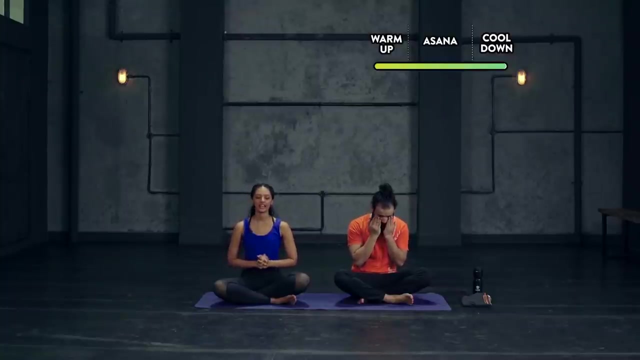 So with that emotion of sincere gratitude, let us end today's session with an Aum and three Shantis. so now take a deep inhalation inwards, inhale Aum And now bring your palms together, chest, rub them to create some heat energy and if you feel like you can place your palms on the eyes, otherwise you can stay here. it's your choice. hands on the eyes, release and exhale.